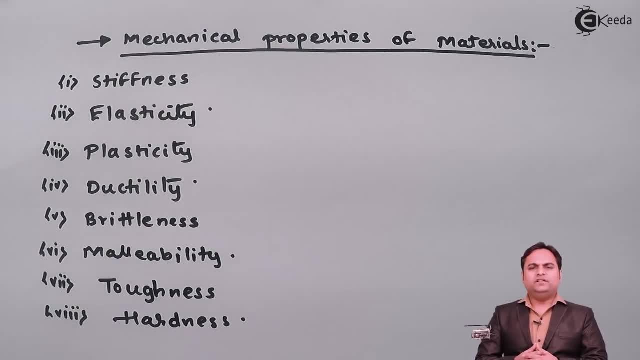 also, we need to learn some basic mechanical properties so that we can understand the behavior of some materials. So here, as I have mentioned, we would be dealing with these properties in detail and we need to have the deep knowledge of them So that we can understand the behavior of some materials. 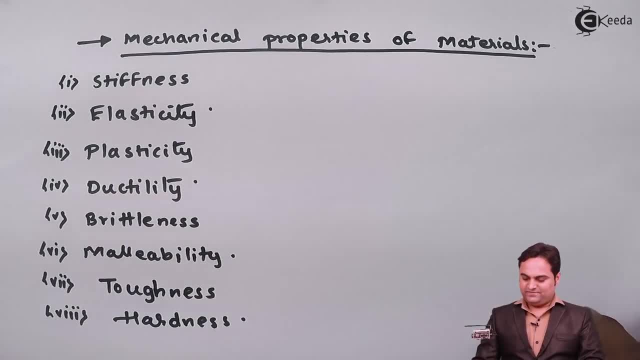 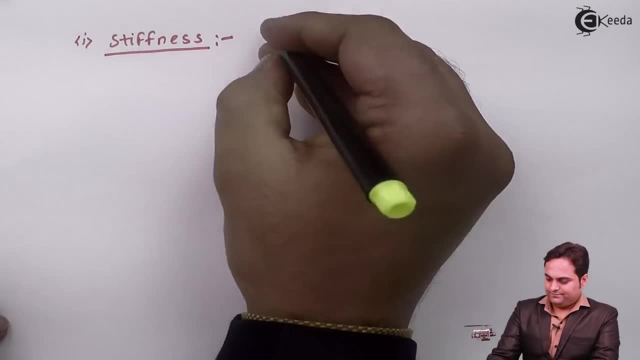 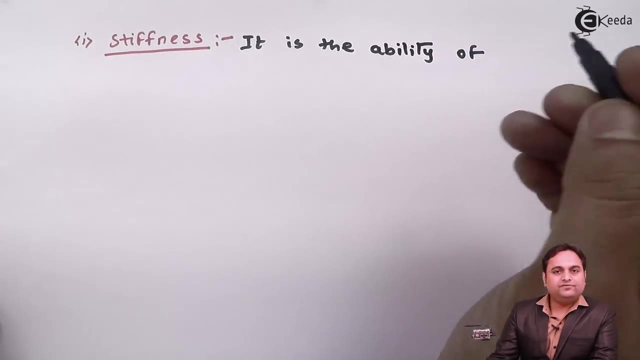 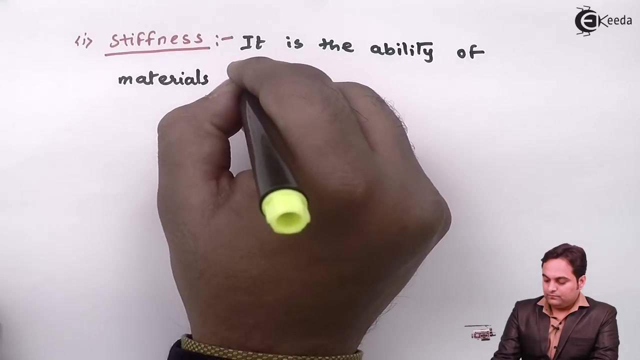 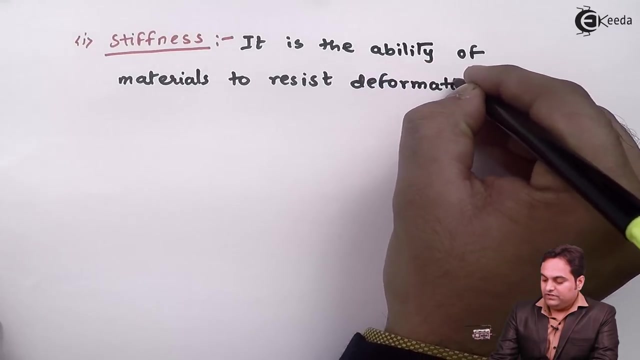 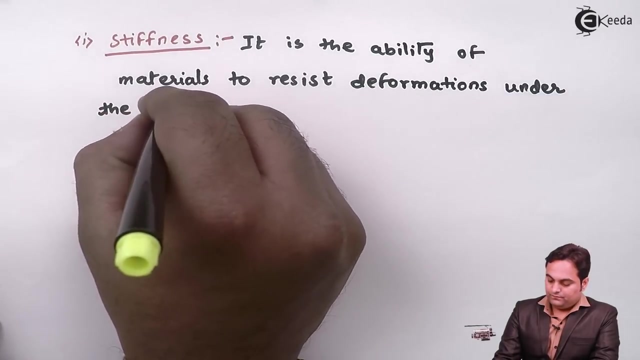 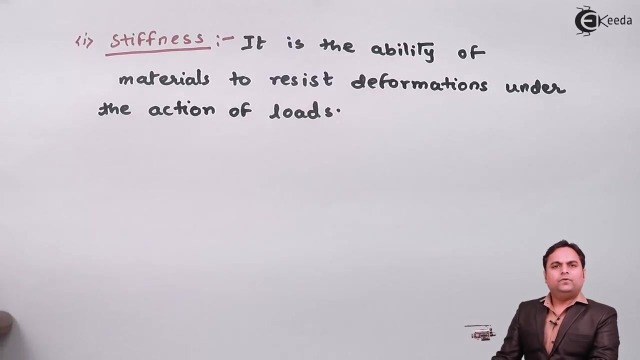 Now let us get started with the first property, that is called as stiffness. Now, stiffness is? it is the ability of materials to resist deformations under the action of loads. So this is stiffness: that it will be the ability of any given material to resist deformation, that is. 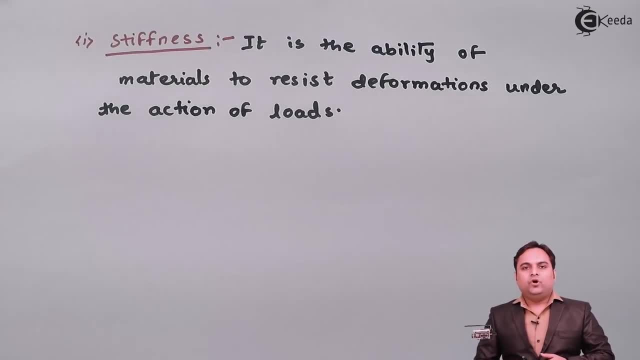 a material should not change, change its shape when the load is applied. and when we go on increasing the value of load, then the deformation should be very, very small. it should not increase with the increase in load. like, for example, if i can say that if the load is 10 newton then the deflection 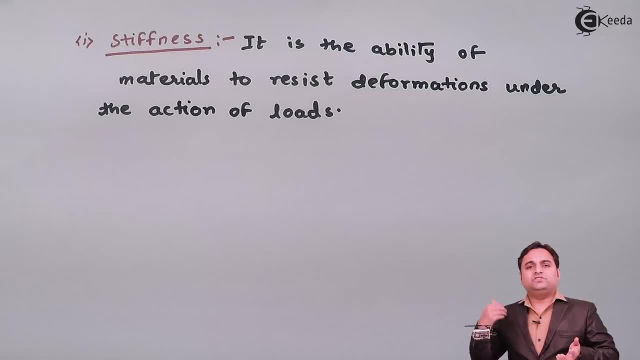 is around 1 mm. if it is 20 newton, then the deflection becomes 10 mm. so it should not be like this. the deformation should be slow. that is the meaning of stiffness: you go on increasing the load value, but the deflection is less so. here i have written about stiffness. 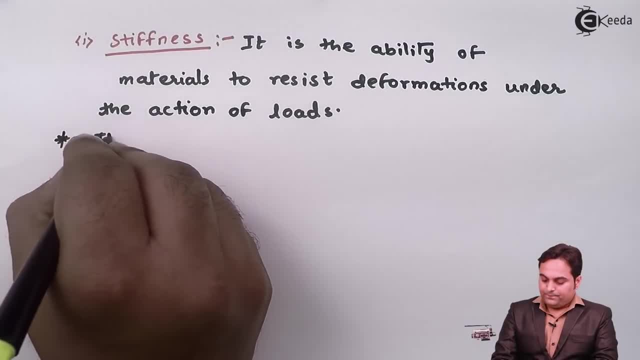 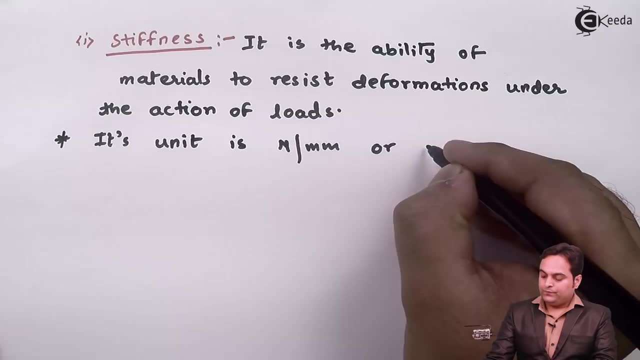 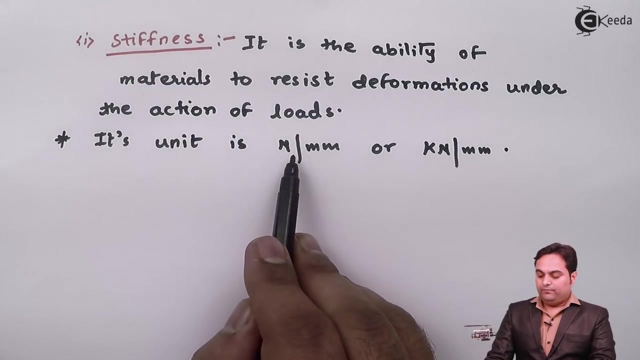 and next its unit. its unit is newton per mm or kilonewton per mm. it is load to produce per unit deflection. that is, in order to produce a deflection of 1 mm, how much load should be applied, that is, in terms of newton or, if it is in terms 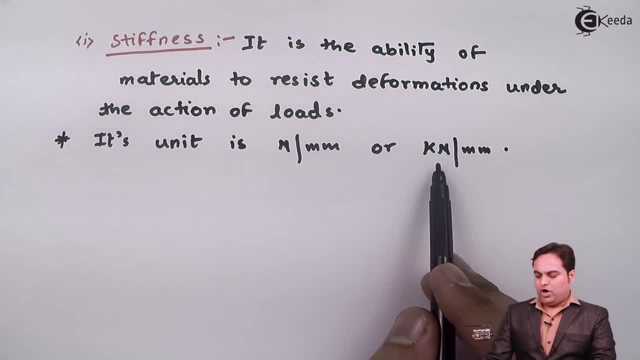 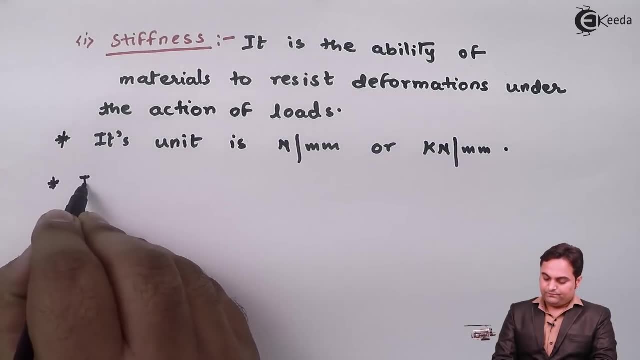 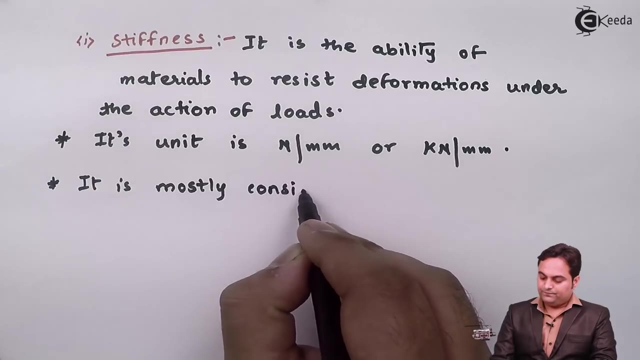 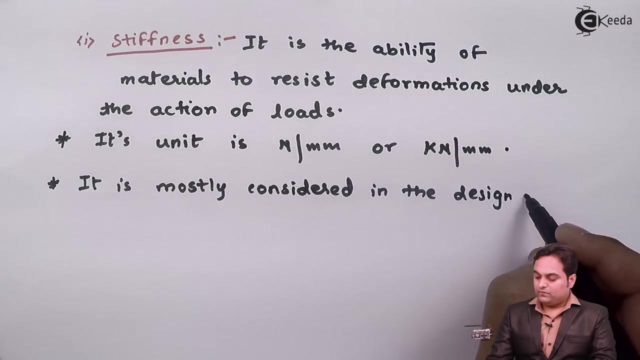 of kilonewton then again to produce a deflection of 1 mm, how much load in kilonewton should be applied? so that is the meaning of stiffness and it is mostly considered to be a deflection of 1 mm in the design of springs. so a very important property that while we are designing the springs, 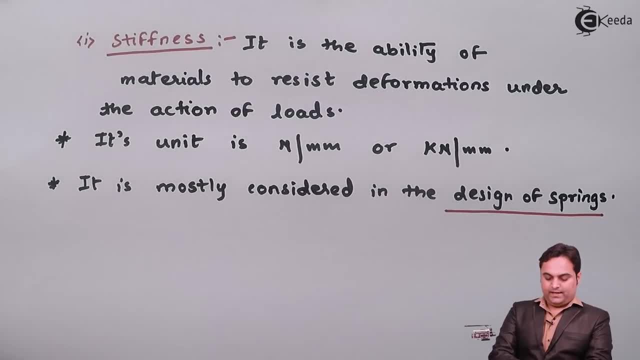 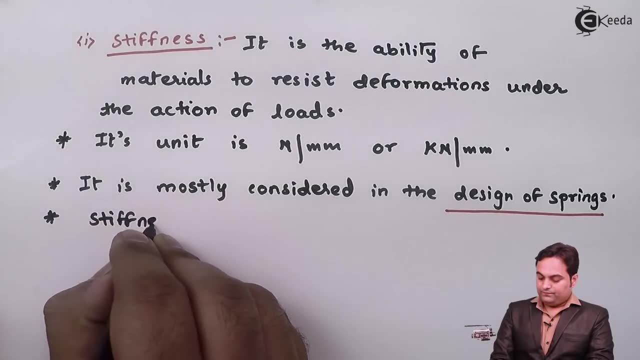 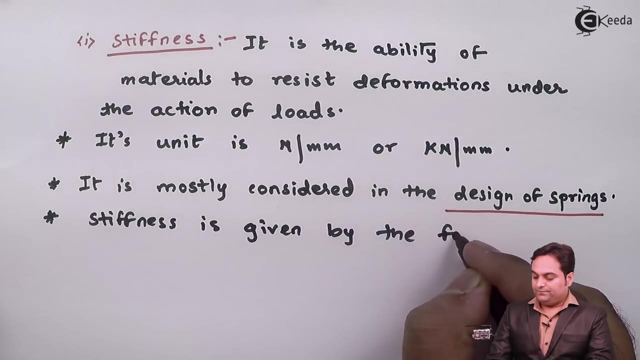 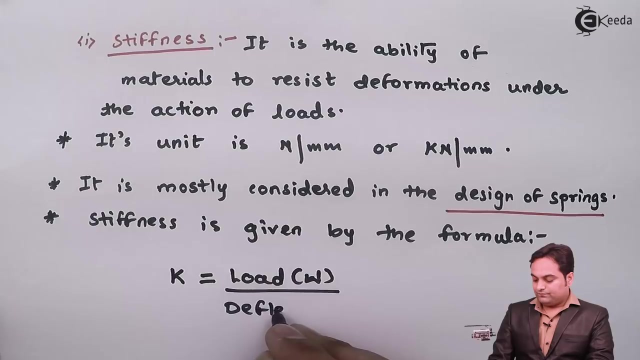 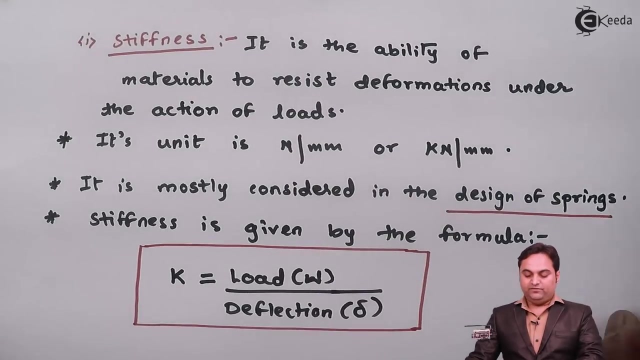 we would be considering the property of stiffness, and here i can say that stiffness is given by the formula here. stiffness, i will denote it by k, and that is equal to load, which is w, upon deflection, deflection is delta. so here is the formula to calculate stiffness. now, after stiffness, the next property which we have. it is called 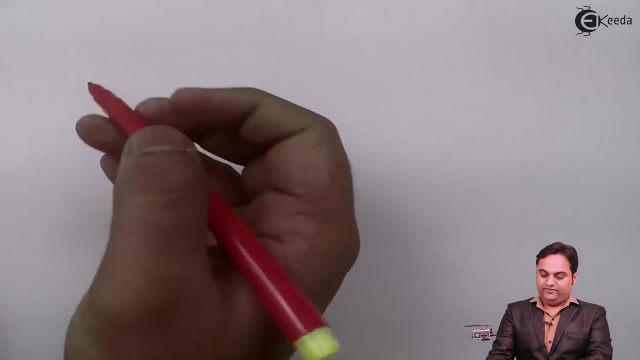 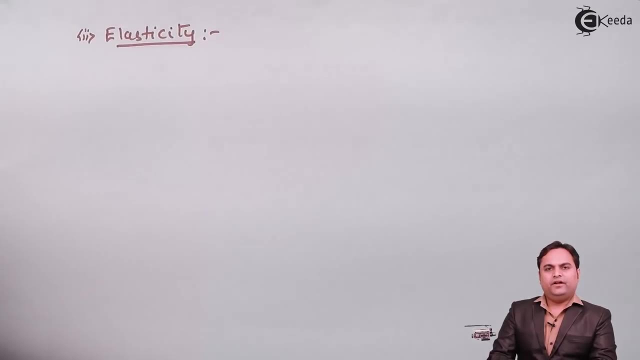 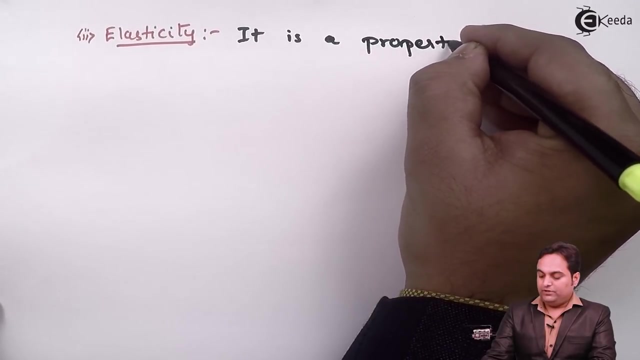 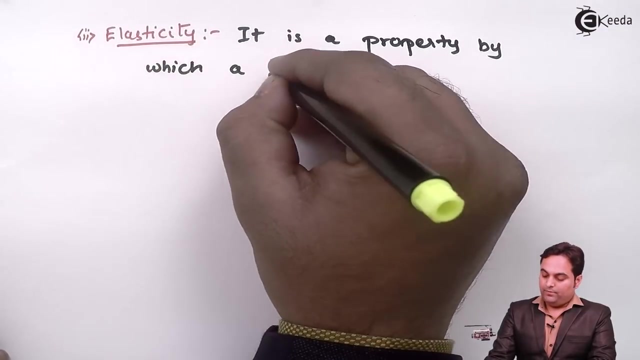 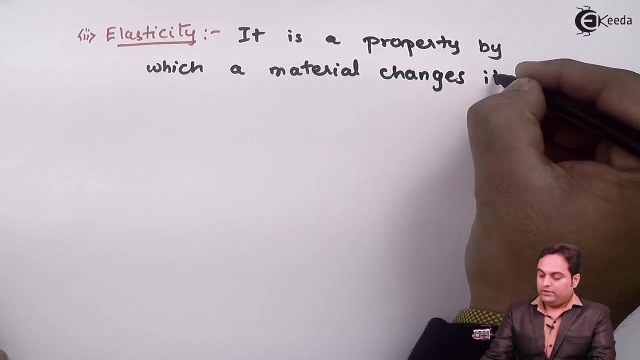 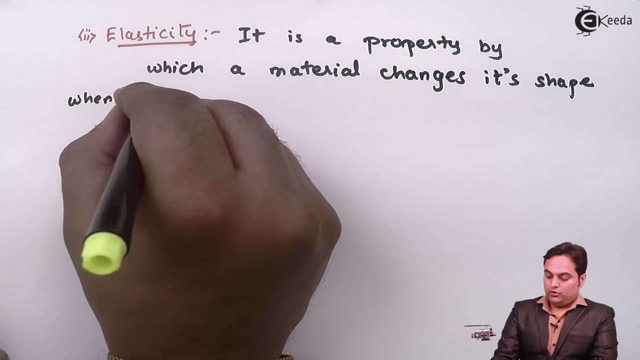 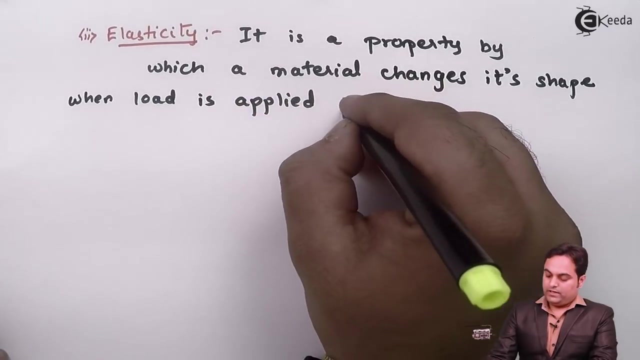 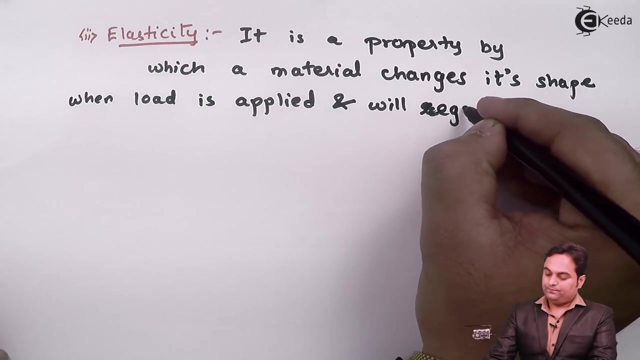 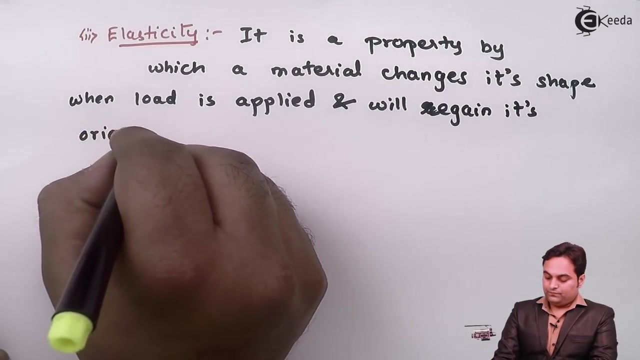 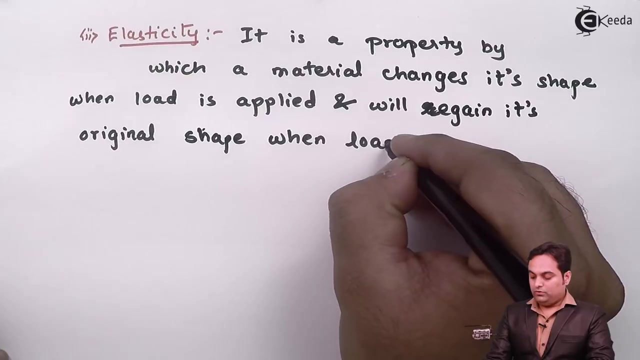 as elasticity. i will define elasticity here. elasticity, it is a property. its a property by which a material changes its shape when load is applied and will regain its shape when the load is removed. it's original shape when load is removed. so this is the definition of elasticity. it means 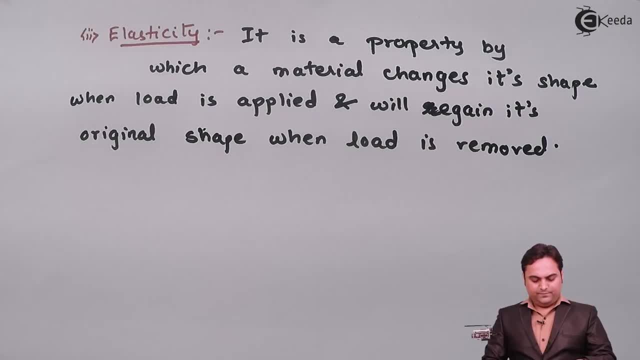 when we apply load like form example. here i have this pin. if i am applying a load over Weg steering on this pin, i am applying load over this pin wed setting method. let us go our first procedure over this. if I am pulling this pin, then its shape will change and the moment I 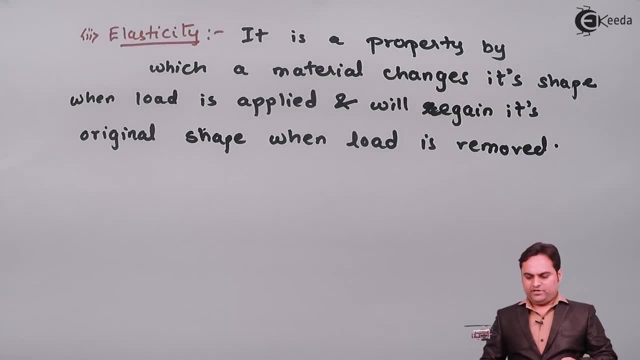 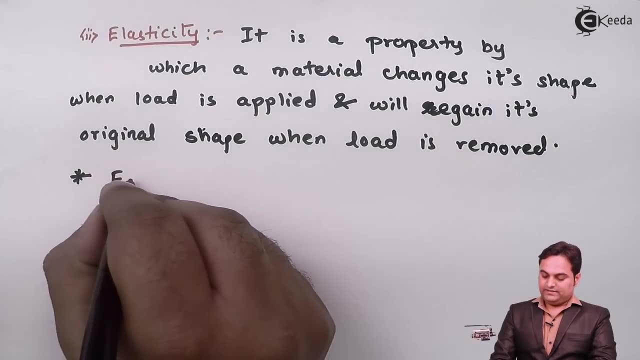 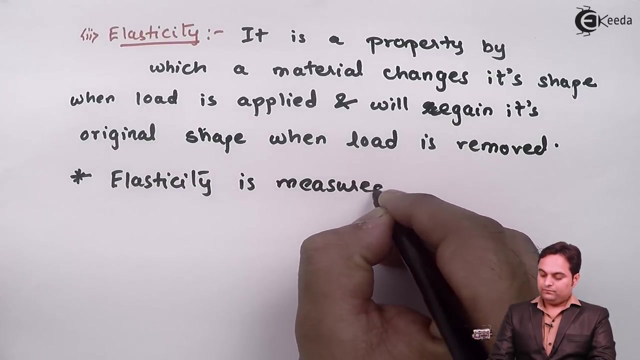 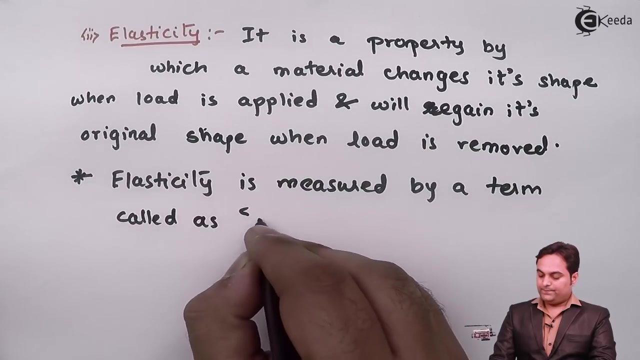 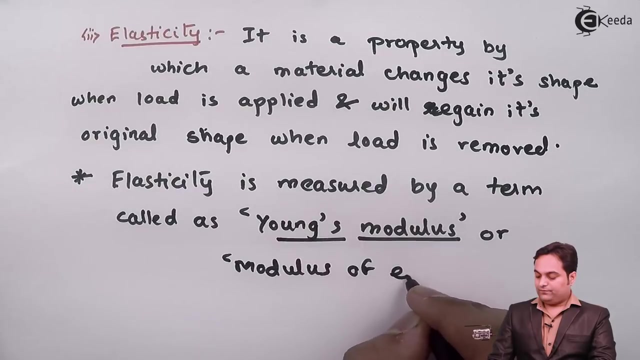 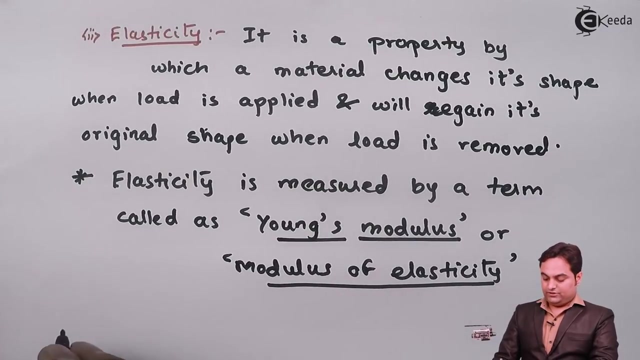 remove the load, it will come back to its original shape. that is the meaning of elasticity. Elasticity is measured by a term called as Young's modulus or modulus of the force. Modulus of elasticity and its unit will be given by. its unit is Newton per mm. 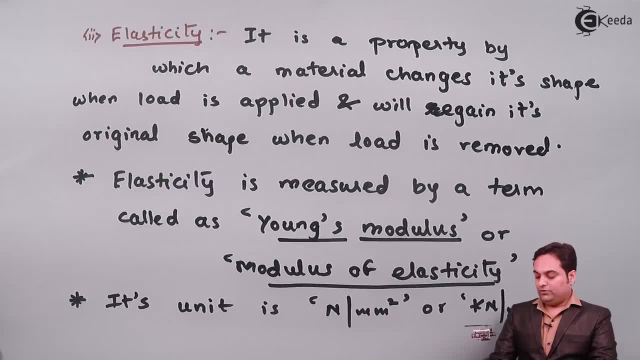 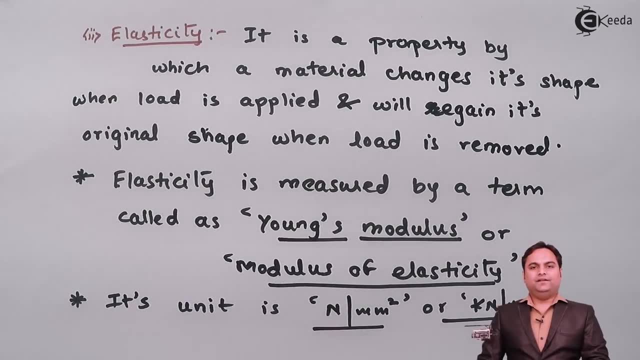 square or kilo Newton per mm. square. So this was regarding elasticity. Young's modulus decides how much elastic a material is. For example, if Young's modulus is very high, it means the material is very elastic. If Young's modulus is value is less, it means that 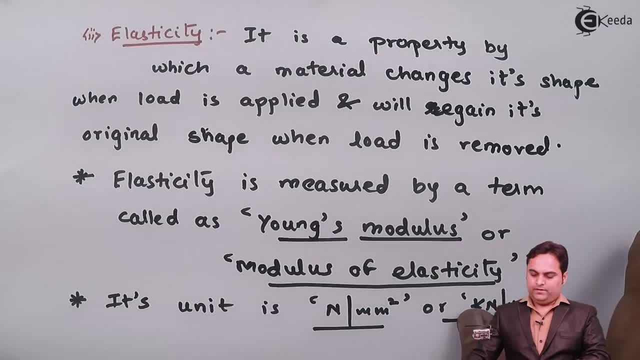 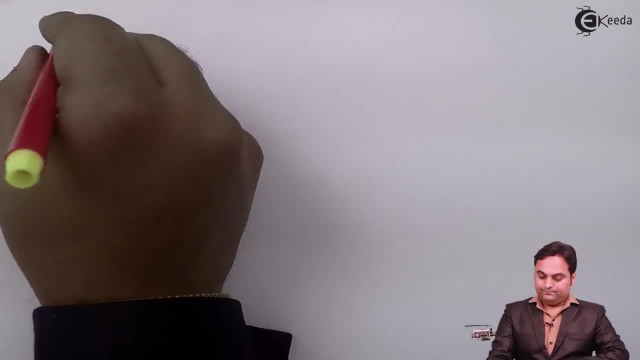 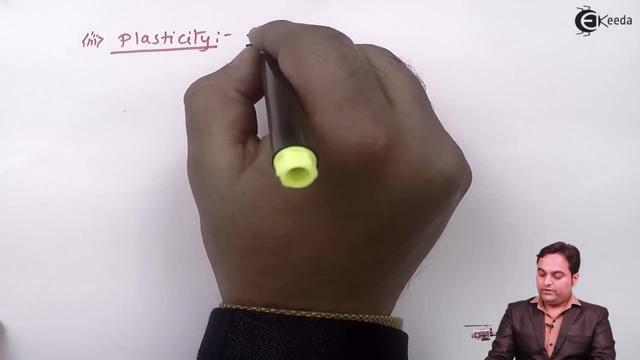 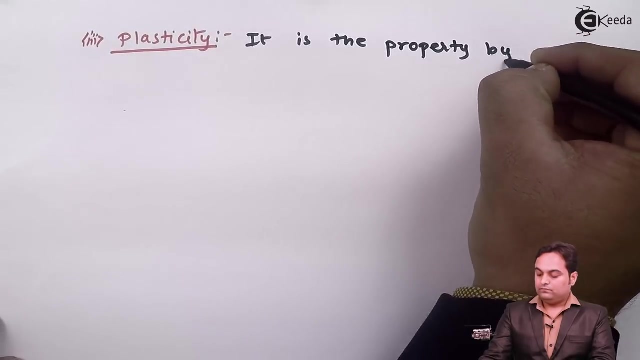 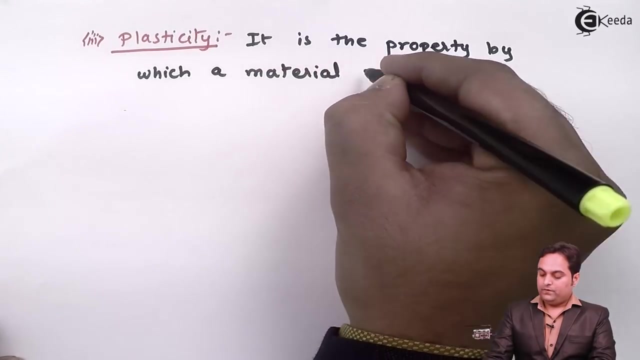 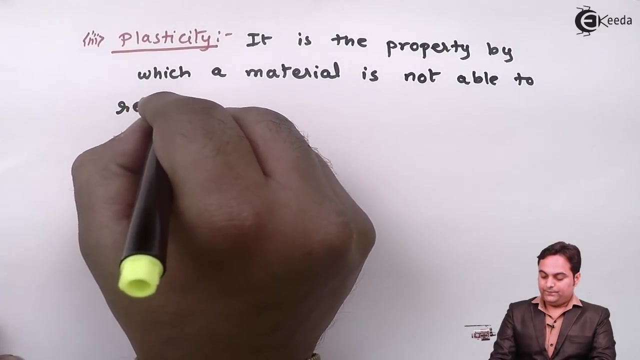 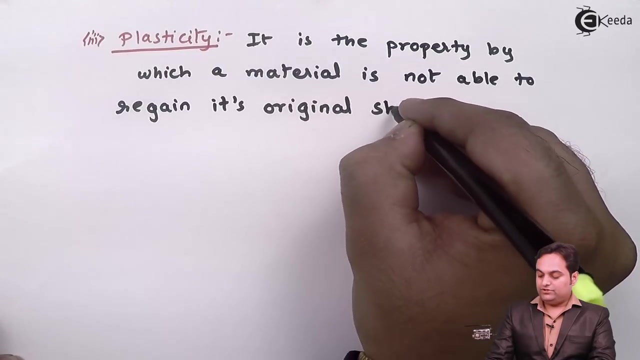 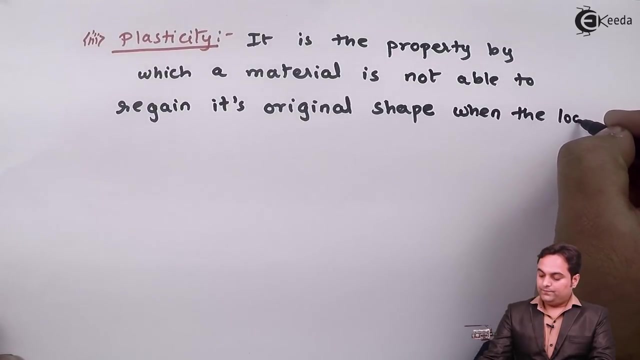 material will behave in a less elastic manner. After this definition, we have the next property, which is called as plasticity. Now, plasticity, it is the property by which a material is not able to regain its original shape when the load is removed. It means here, in case of 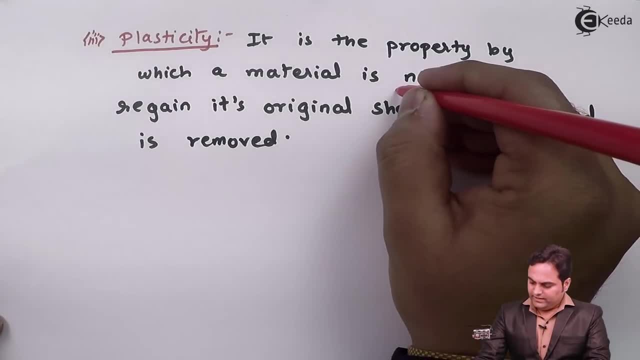 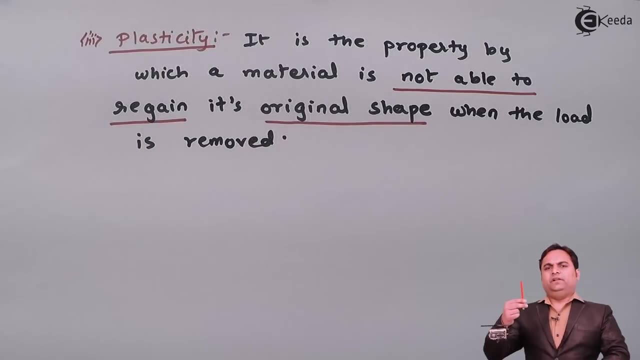 plasticity the material will not gain. it is not able to regain its original shape, Like, for example, I have this pin. if I am applying a load and pulling this pin, Then its shape will change and the moment I remove the load it will not regain its original shape, Means when the load was applied, the shape has changed. 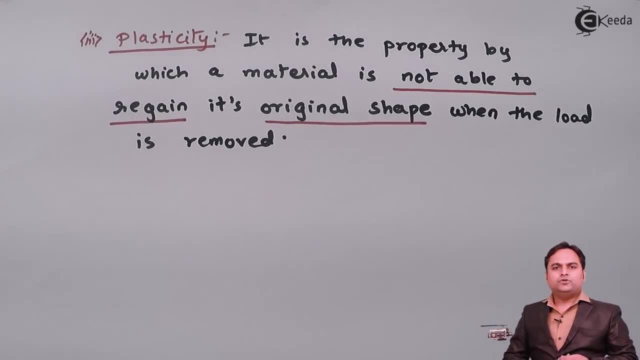 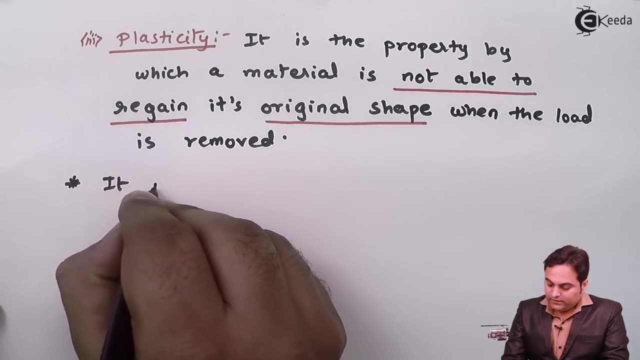 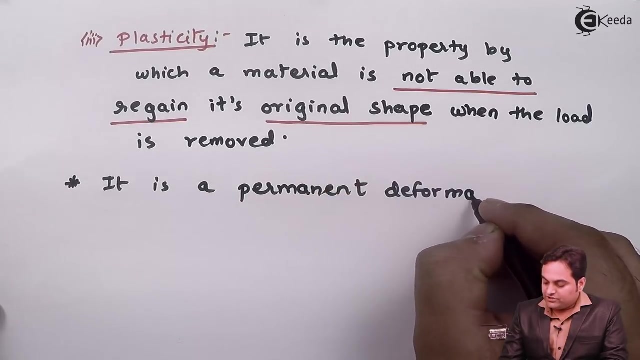 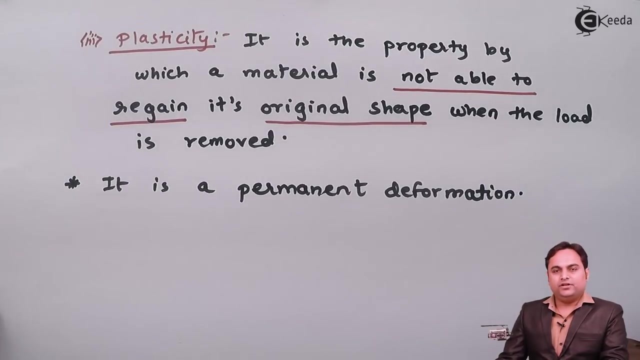 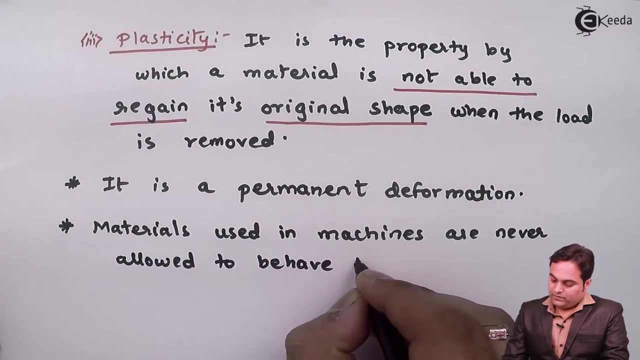 that change in shape will remain permanently. So we have understood that plasticity is nothing, But it is. It is a permanent deformation, as the material is unable to regain its original shape. so it comes under the category of permanent deformation. Most materials used in machines are never allowed to behave in a plastic manner. 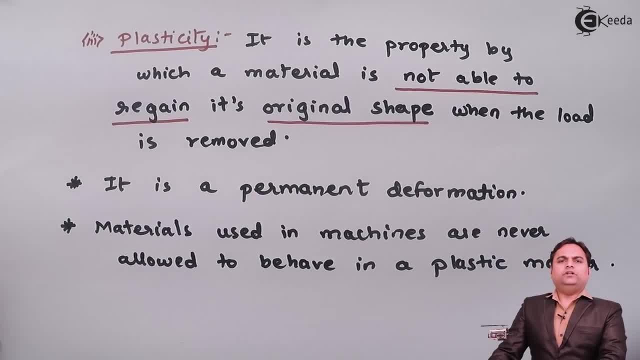 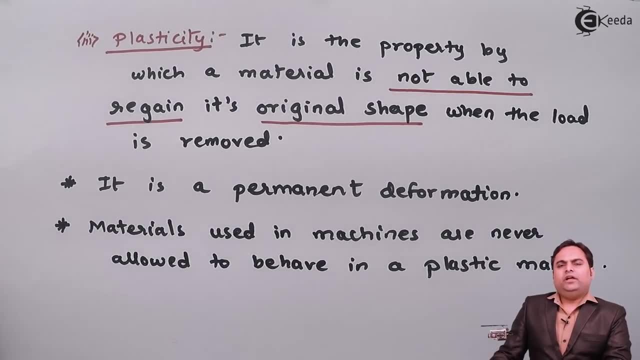 This is a very important consideration. like whatever materials we are using for machine design, that materials- they should not operate in a region where the deformation would be plastic, that is, they are not allowed to behave in a plastic manner. It means, whatever machines we are seeing, they are designed on the concept of elasticity. 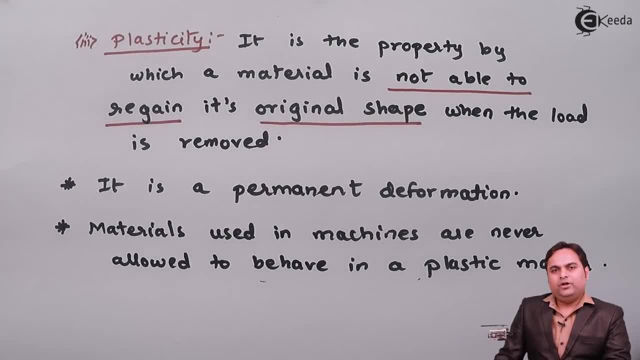 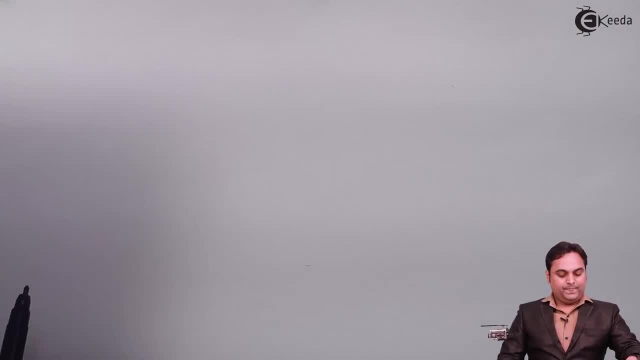 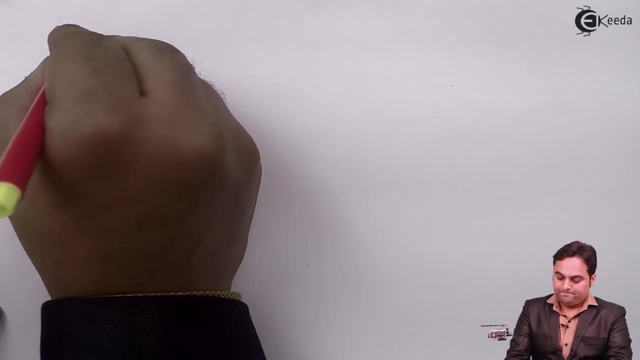 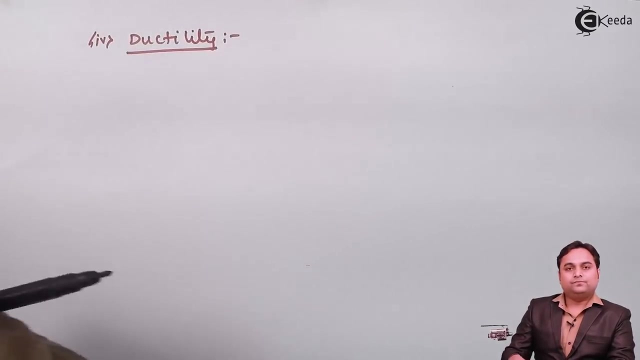 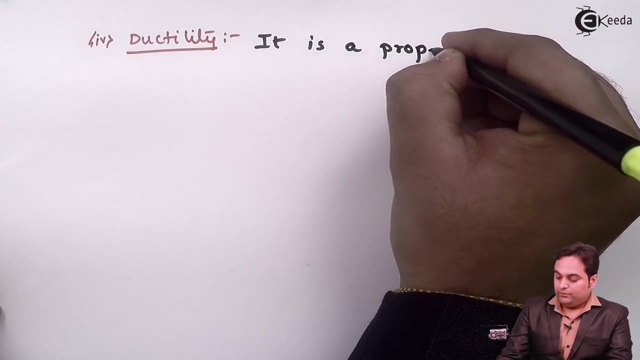 that is, they should regain their original shape when the load is removed. They should not behave in a plastic manner. So next, after this, the next property which I have here: mechanical property. it is called as ductility. Now, ductility, it is a property. 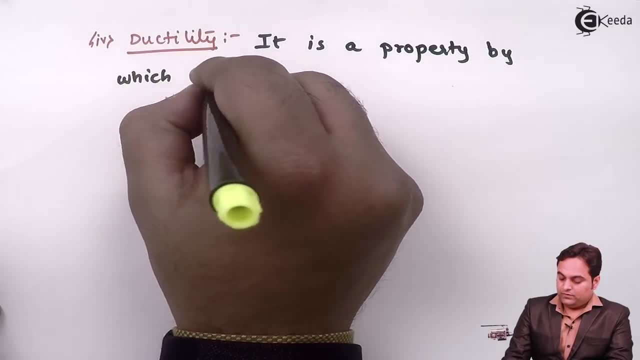 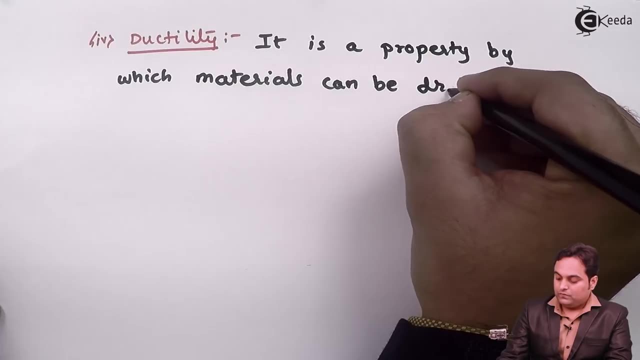 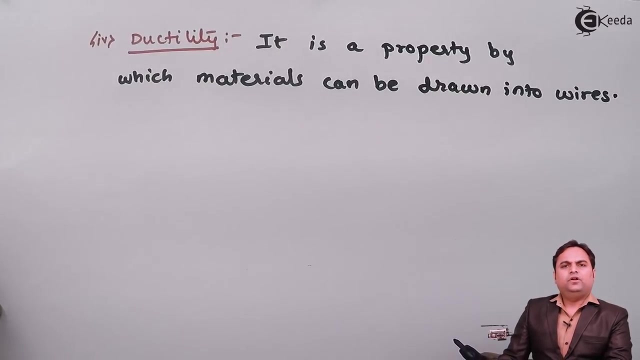 By which materials can be drawn into wires, a very important property, that if a material is having ductility, it means it can be drawn into wires. now, whatever wires we are seeing, like The electrical connections, those wires, the material with the help of which they are made, 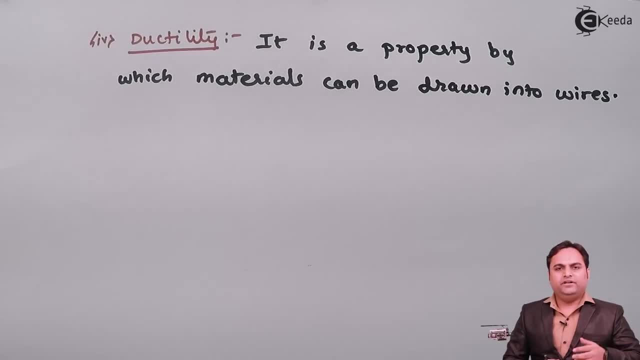 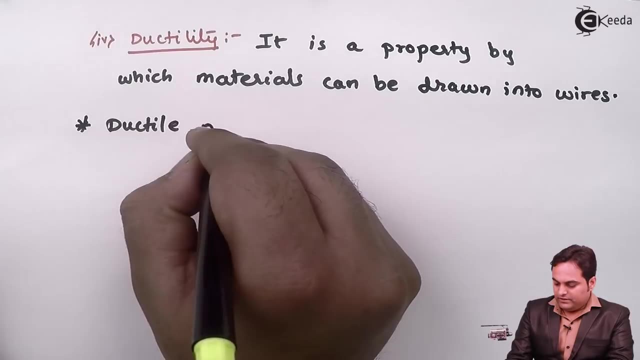 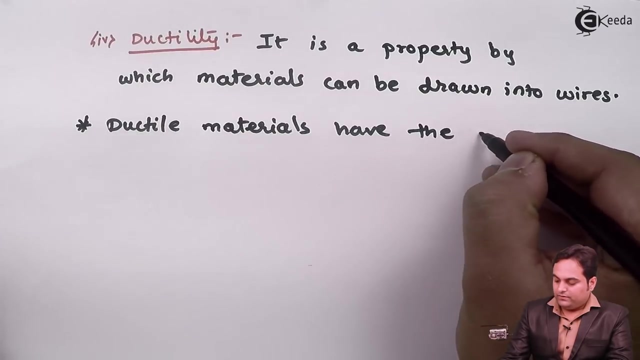 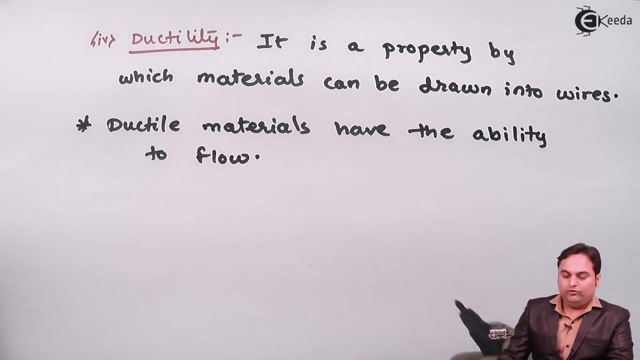 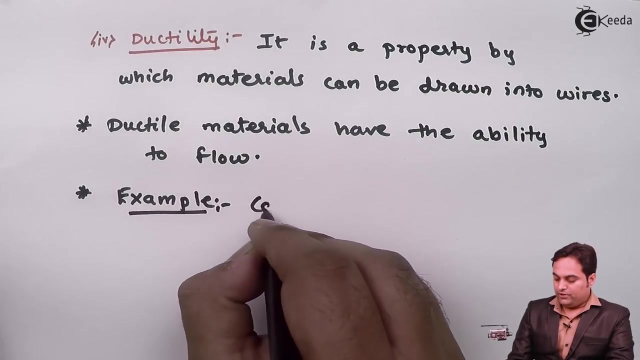 that is that material. it is called as a ductile material. So here I can say that ductile materials have the ability to flow. To flow means when the load is applied the material will elongate. it will change its shape. Example: copper wires used in electric cables. 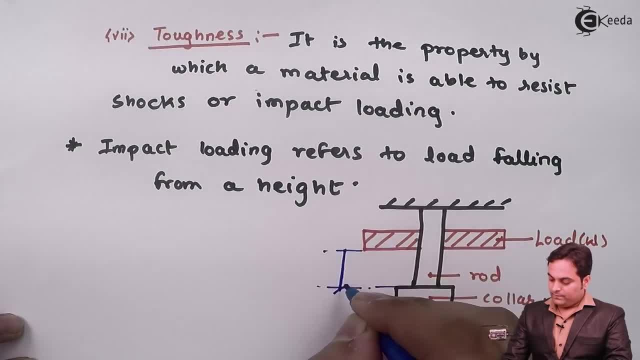 Now here I have height h, through which the load is falling onto this collar. So now, toughness means the ability of this collar to resist this load. Like, for example, if this load is falling through this height h, then this collar should not deform much. By toughness we mean that on the application of this load, this collar should be able to resist this load. 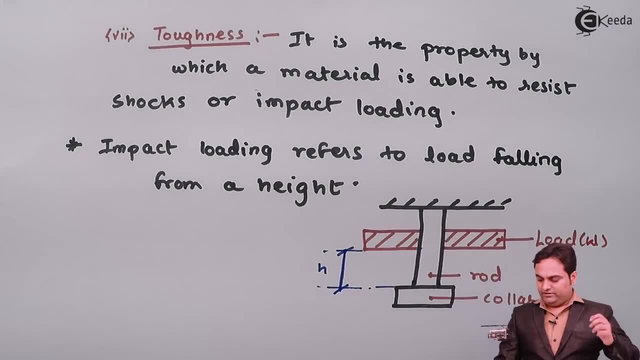 It should not go or it should not deflect suddenly. The deflection should be minimum. If I can draw the diagram that after deflection it will look something like this: So this much is the amount of deflection, which is delta L. So a material which is able to resist impact load means if a load is falling from a height, then that is called as toughness. 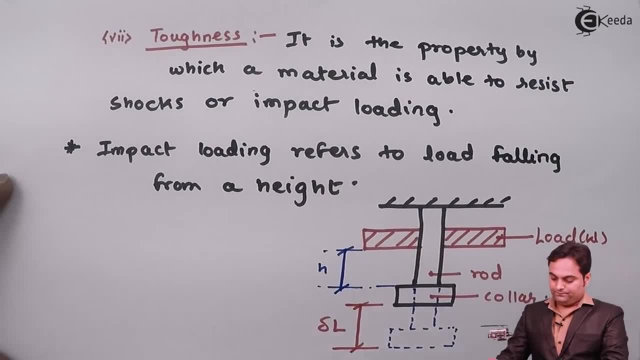 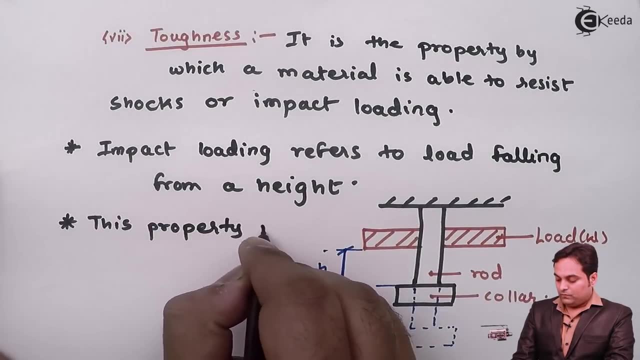 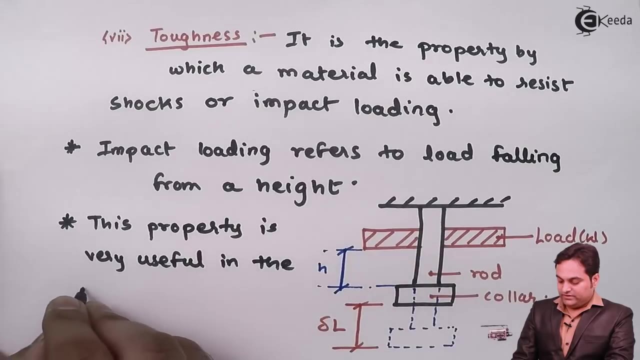 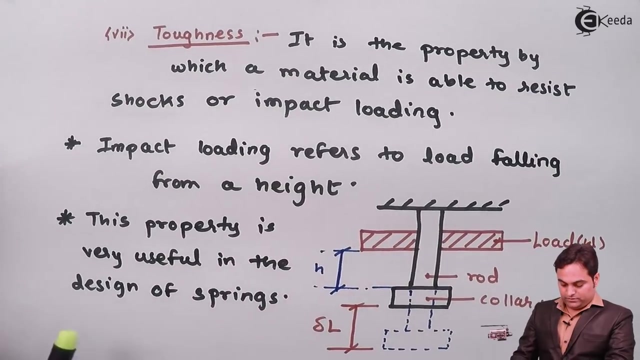 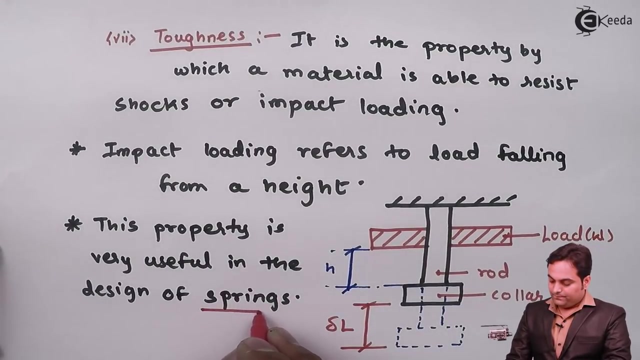 And this property. This property is very useful in the design of springs. Like previously, we have seen the property, which was The property which we have seen, That was Stiffness. So stiffness is required in the design of spring. at the same time, toughness is also considered, while the design of springs. 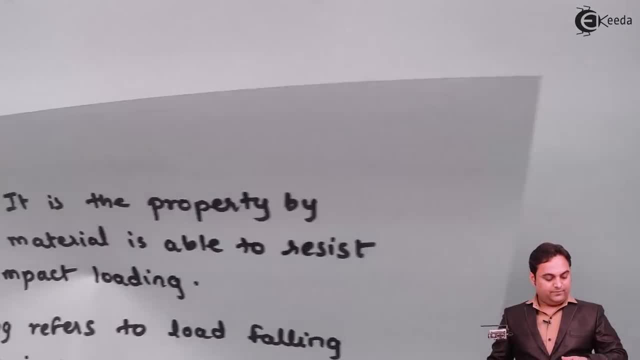 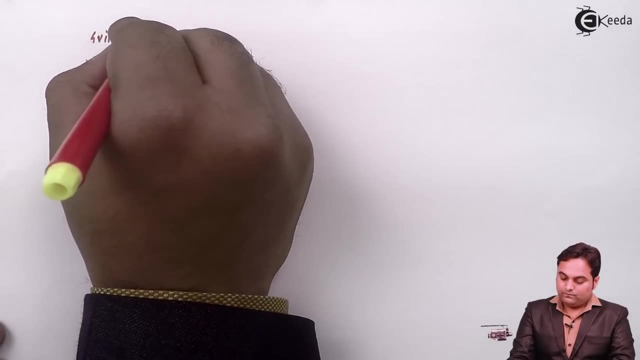 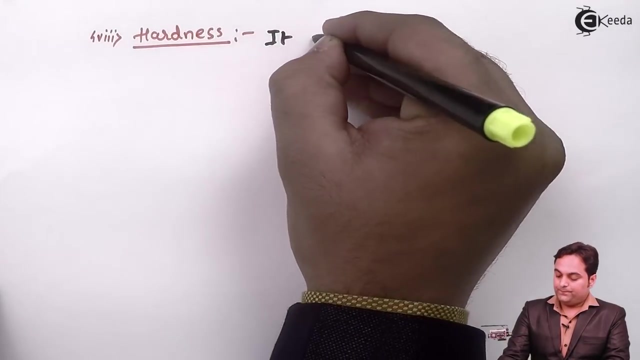 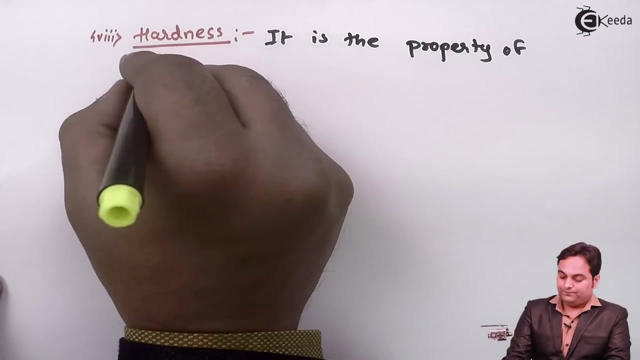 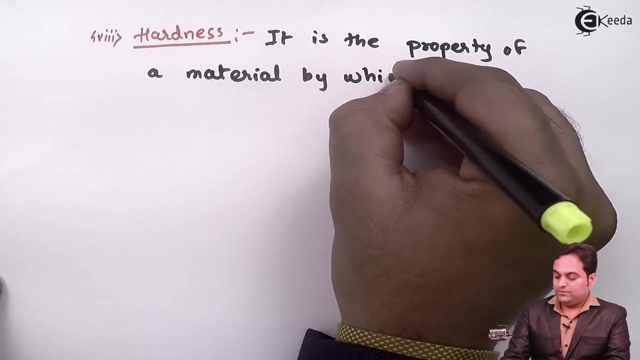 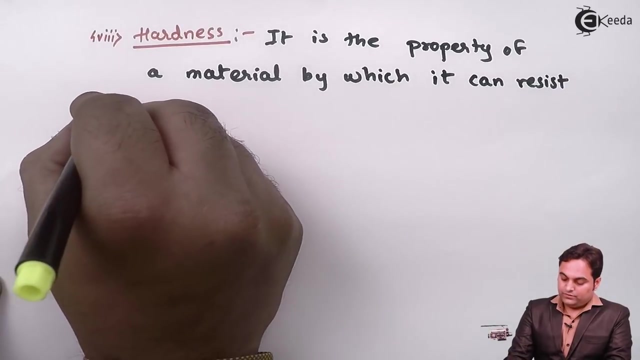 So I hope toughness is understood. next we have the property which is called as hardness. Hardness is the opposite of toughness. Here I'll mention It is The property Of A material By which It can resist Scratches. 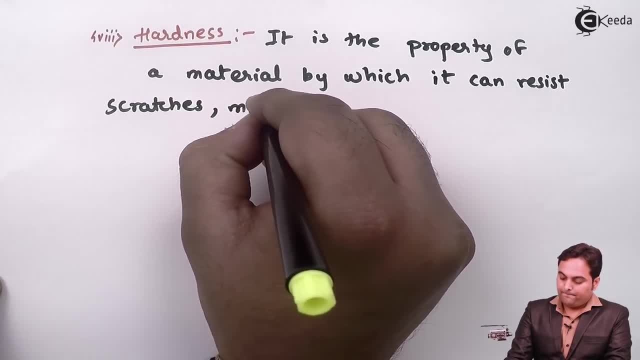 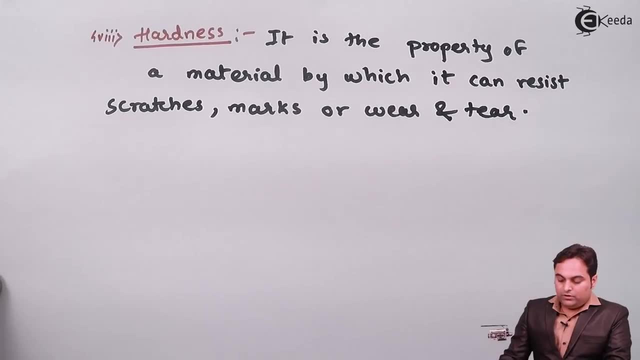 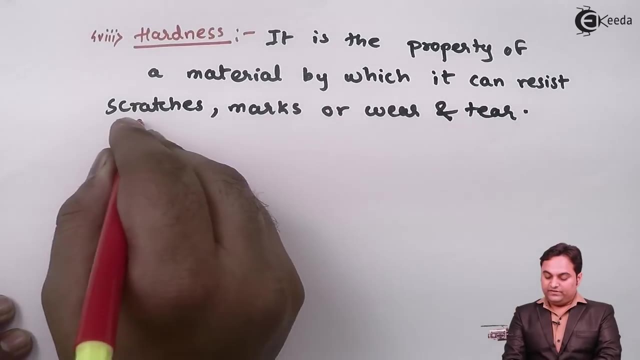 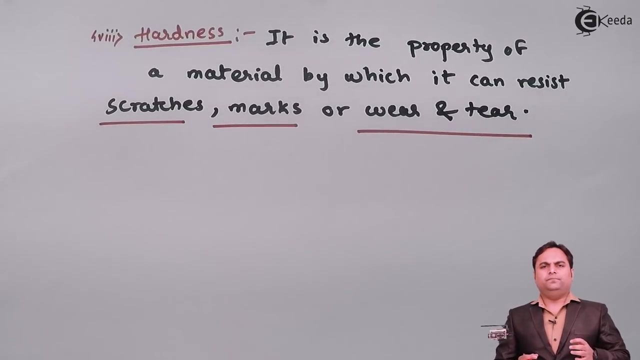 Marks Or Wear and tear. So This is regarding hardness, that it is the property by which material is able to resist scratches, marks or wear and tear. See, we consider, we decide the hardness depending on the ability of the material. Hardness is independent. 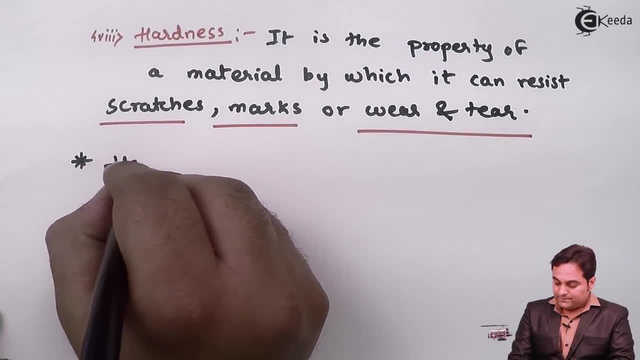 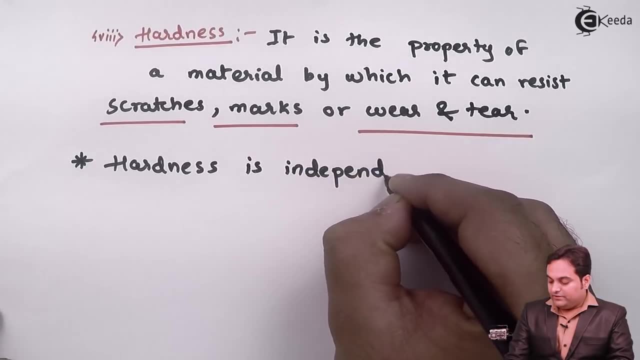 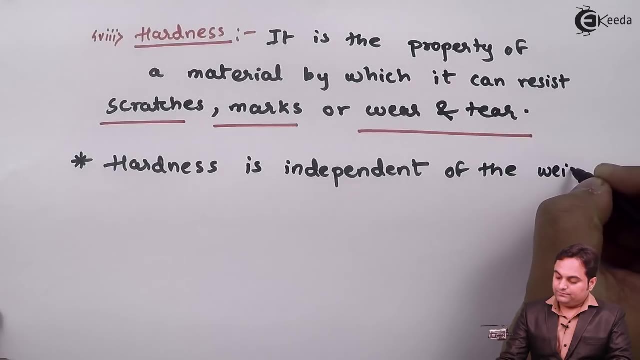 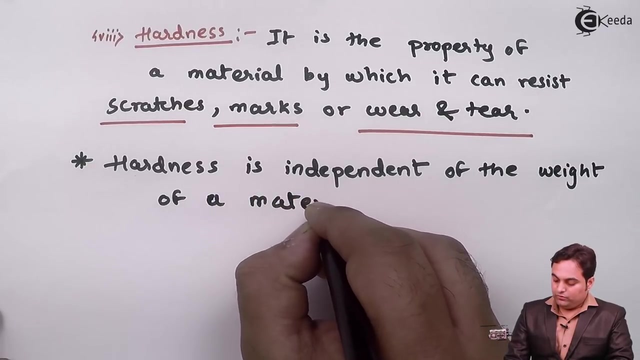 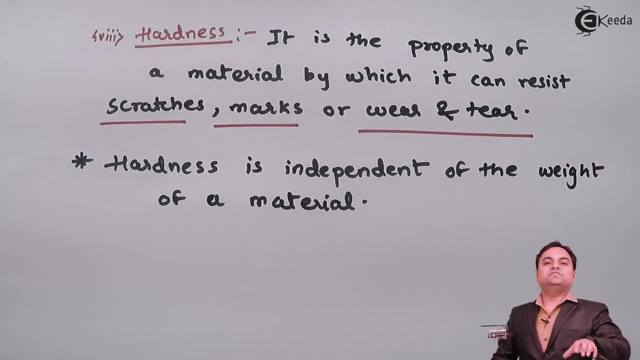 I'll mention here: Hardness Is Independent Of The weight Of Of the weight Of A material. So we cannot say that if a certain material is heavy it means it will be hard. If a material is light, then the hardness will be less. 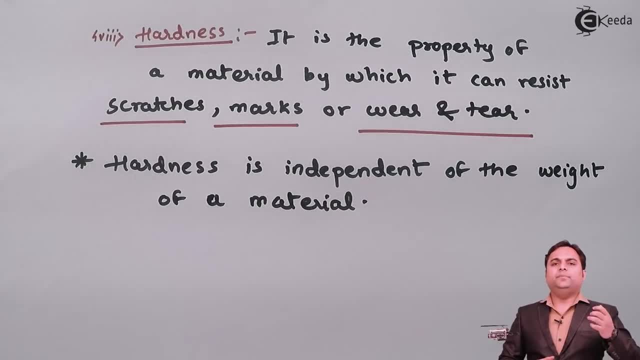 We cannot say this Because hardness is independent of the weight of the material. And Like for example, and like for example, here I have this two different color pin. if I want to decide their hardness, then I would be scratching, I would be marking on each of the pin and, if I am able to, 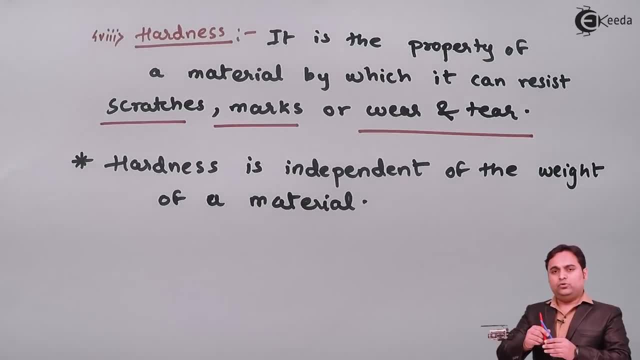 mark very easily, or I can able to scratch, for example, this red pin. if I am able to scratch this easily, it means it is less hard. or if this blue pin. if scratching the blue pin is difficult, it means it is more hard. so hardness is regarding the scratches or wear and tear. 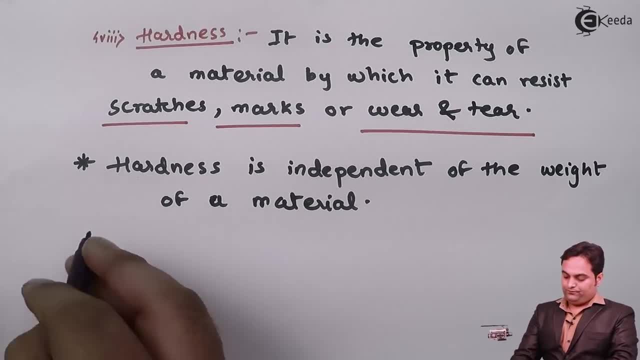 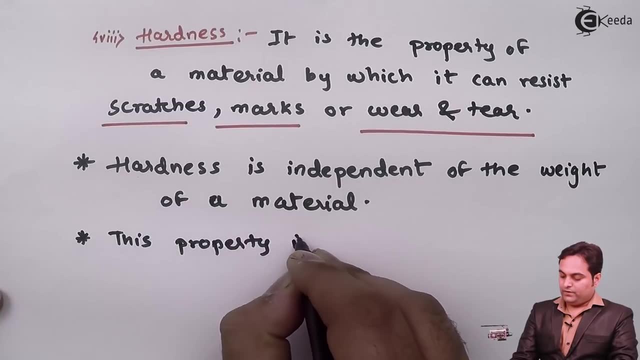 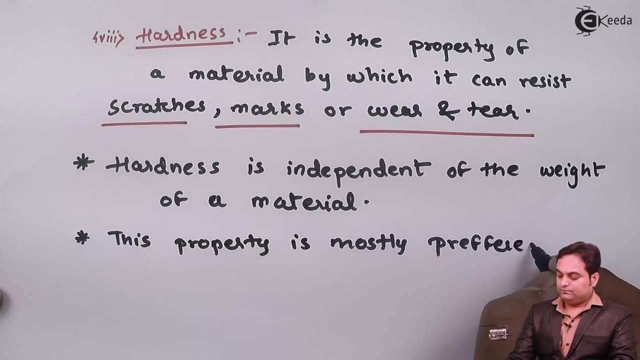 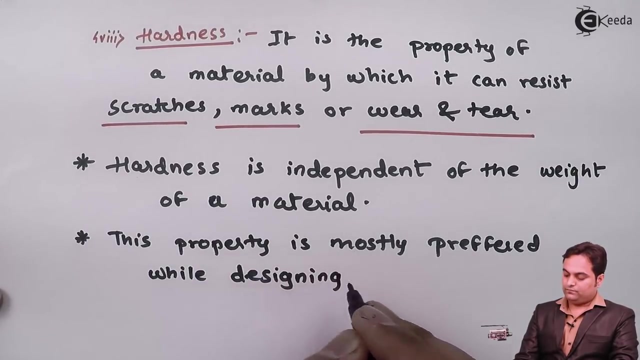 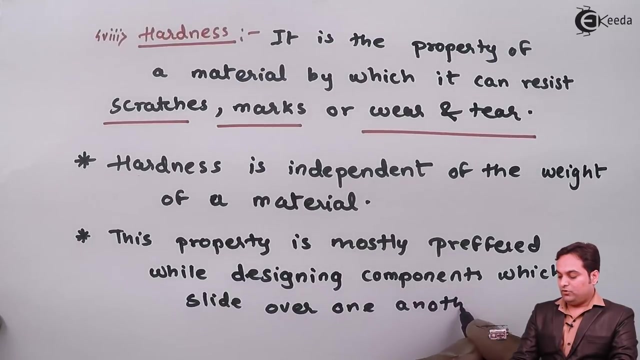 which is produced on the surface. this property is mostly preferred while designing components which slide over one another. so when we have two components and out of that one is sliding over the other, then the surface contact is more and we require hard materials. because if the material is soft and then there is sliding taking place, then there will be more wear and tear. 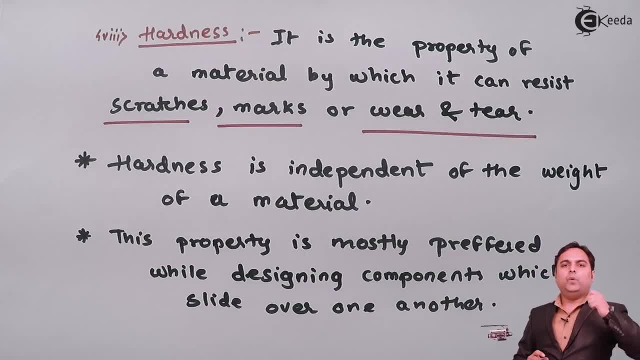 so in case of hard material, we require hard material. and then there is sliding taking place of hardness. we should be aware that the material is hard. it means it should be able to resist scratches and wear and tear. next, after hardness, I can write one more point here. in case of 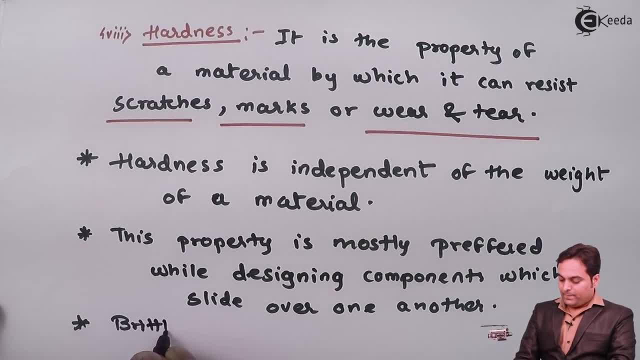 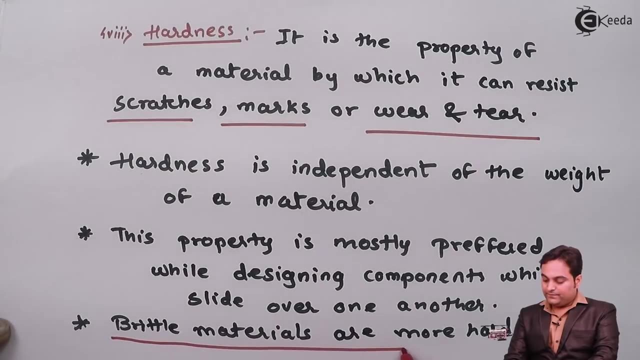 hardness, that brittle materials are more hard. this is a very important point here which I have mentioned- that brittle materials, they are more hard. it means brittle materials are able to resist scratches more like, for example, cast iron. it is a material which has high amount of hardness because it is brittle also, and even we can give the example of concrete. concrete is a 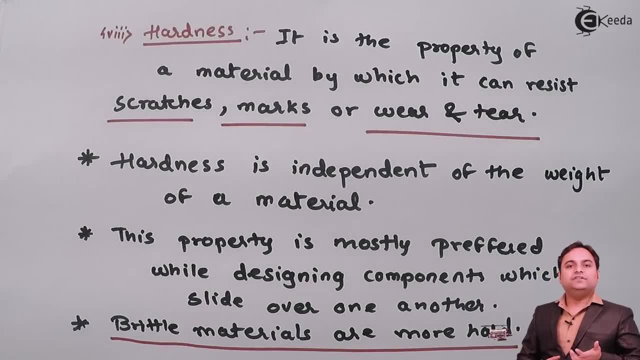 hard material we are unable to scratch it. even glass is an example of a hard material. like we can say that glass is one of the hardest materials which is available. even diamond is an example of a hard material. it is difficult to scratch diamond, difficult to scratch glass. now, 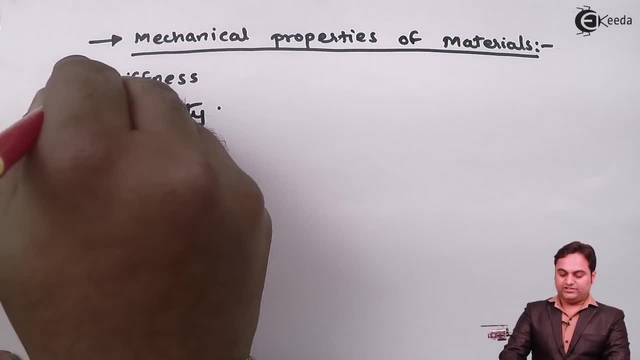 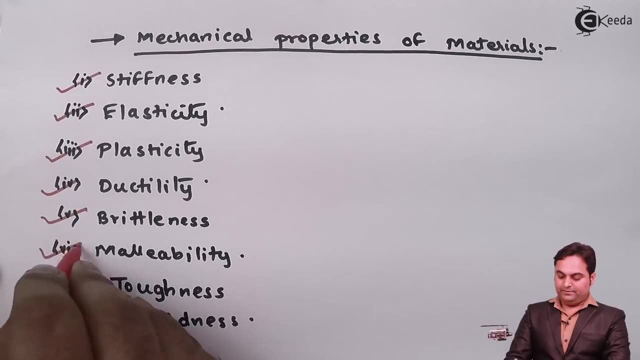 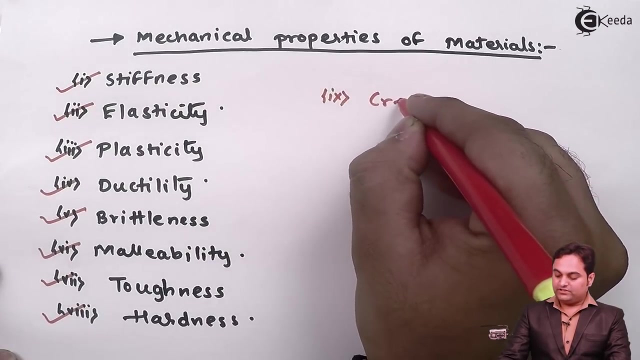 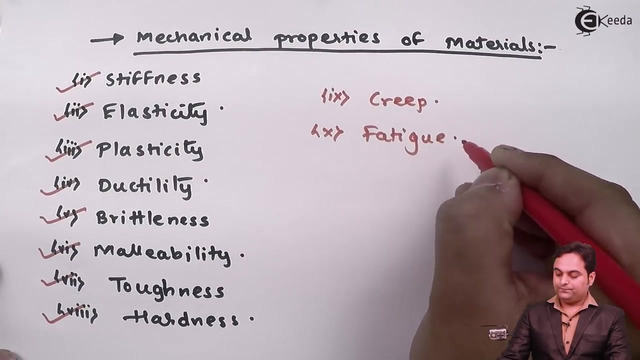 once we have seen these mechanical properties, like we have seen what is stiffness, elasticity, plasticity, ductility, brittleness, malleability, toughness and hardness. here I'll mention two more properties, which is called as creep, and next the other which is called as fatigue. I'll start with creep first. 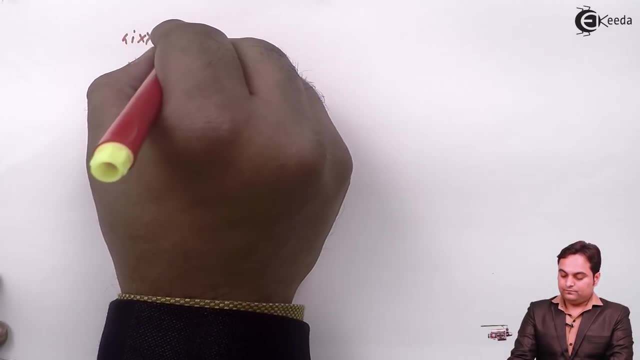 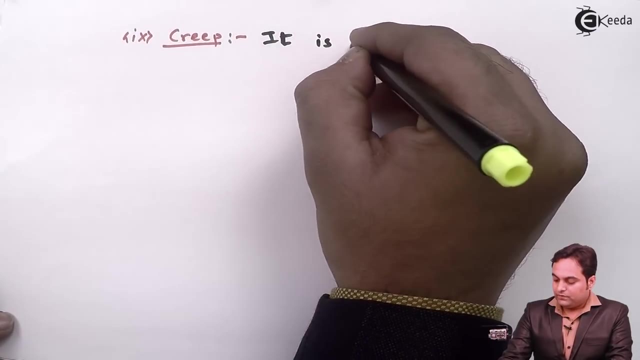 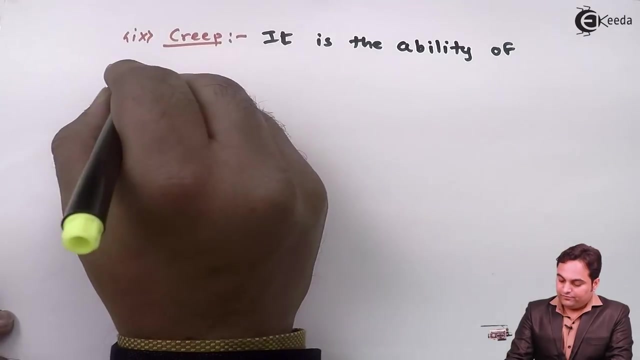 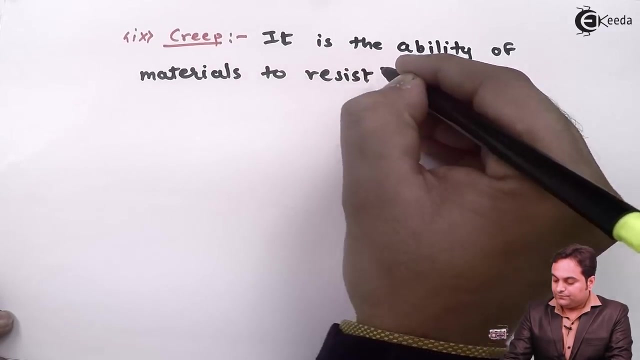 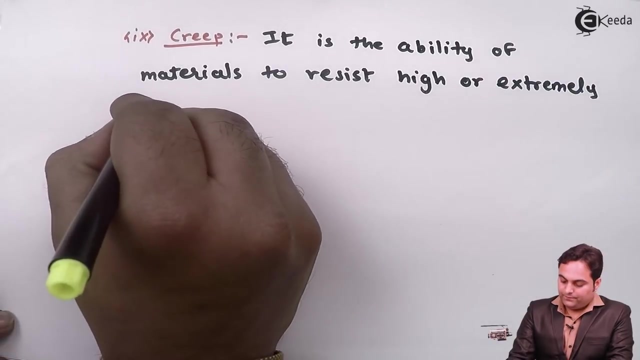 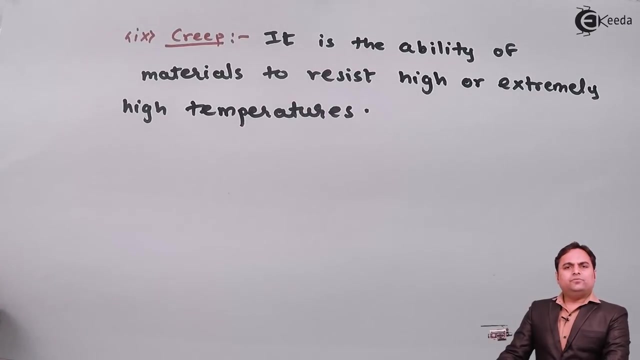 now creep, it is the ability of materials to resist high or extremely high temperatures. so as from the definition, I think it is very much clear that any material which is able to resist high amount of temperature, that material we will say that it is creep resistant, and if the material changes its shape when the temperature is high, then it would be called 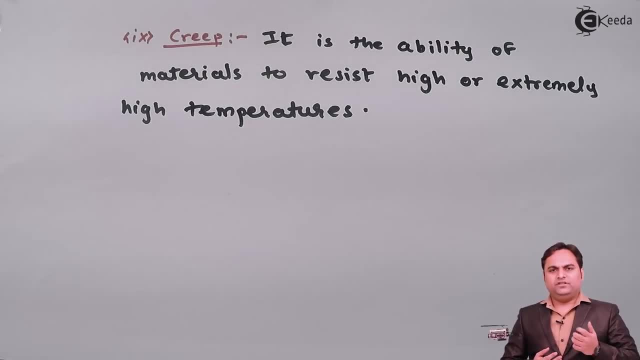 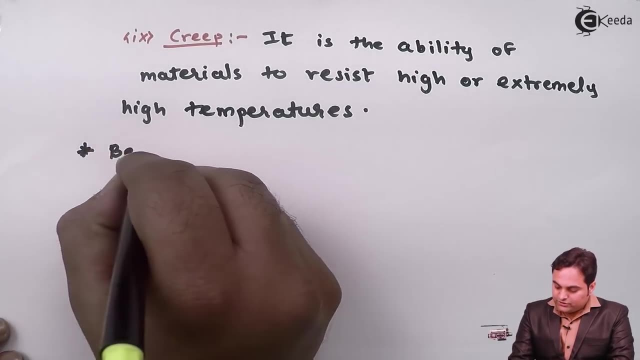 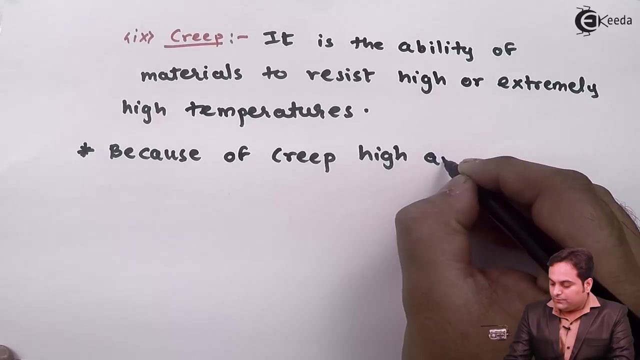 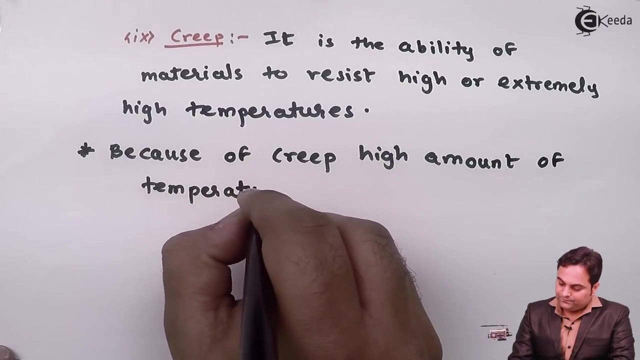 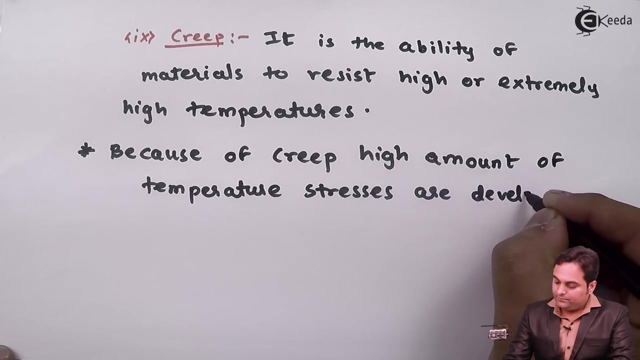 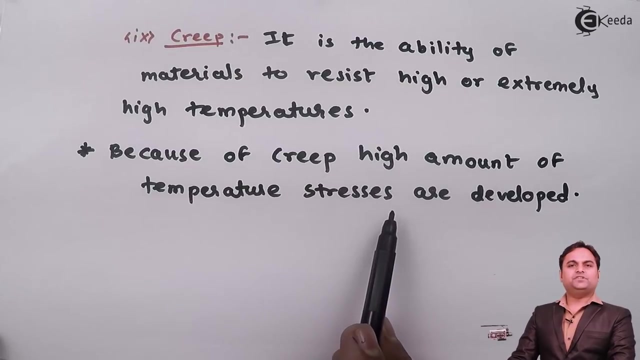 as the material is not able to resist the high temperature, then it would be less in creep. so here I can write down: because of creep, high amount of temperature stresses are developed. A very classic example: like because of creep, high amount of temperature stresses, creep results in the temperature stresses and, as we know, 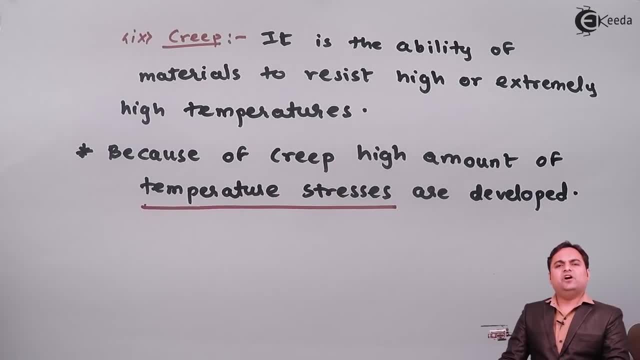 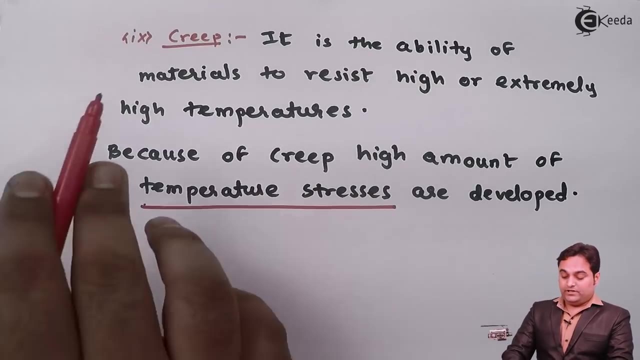 what is the meaning of temperature stresses here? when we have a metal, when we are heating that metal, we know it will expand. because of that expansion there is some stress which is stored in the material and that stress would be called as temperature stress. so creep is the property. I'll write down examples. 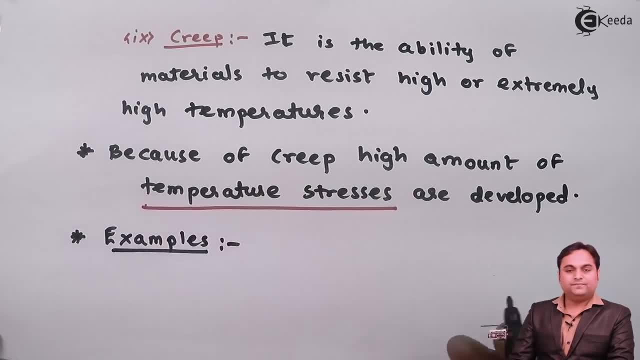 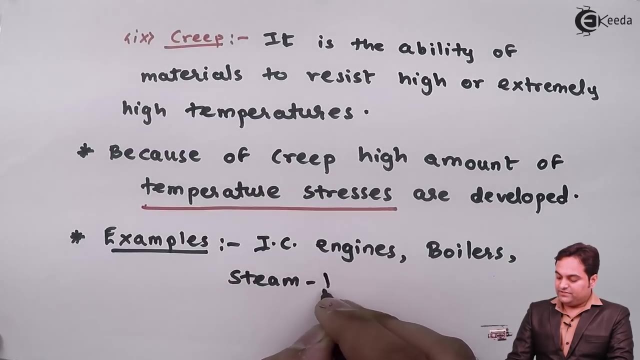 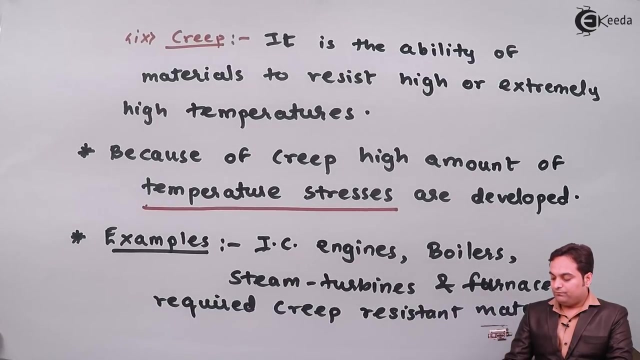 where we require creep resistant materials like IC engines, that is, internal combustion engines. next, boilers, steam turbines and furnaces require creep resistant materials means materials. see, as we can just look at the examples, like IC engine, boilers, steam turbines and furnaces. in all of these we have very high temperatures. we can say from high to. 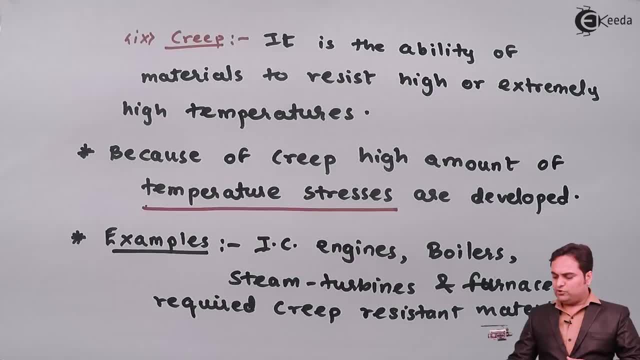 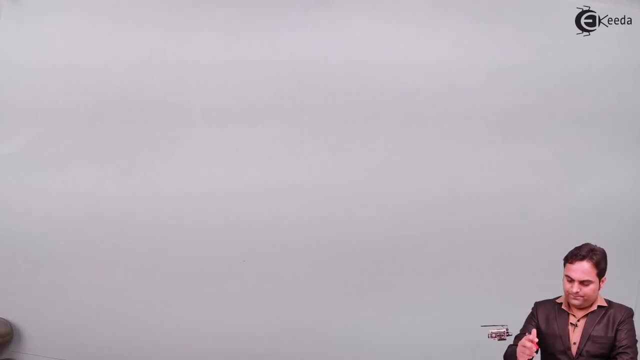 extremely high temperatures. so the materials which we should use in these machines, they should be creep resistant, they should not change their shape when the temperature is high. so this was regarding creep. and last we can see the next property, which is called as fatigue. see by fatigue, I can give you the example, like, for example, I have this pen. 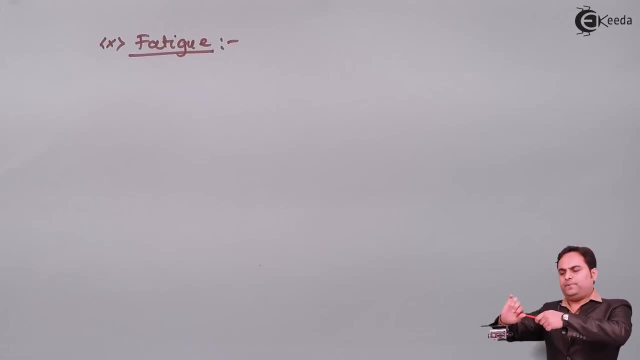 which is red in color. now, if I am twisting this pen from one side and reverse twisting it, that is, I am applying two opposite torques and then I am changing my direction. so suppose, if this material is very thin, then what will happen? because of this continuous twisting, it will break. so here in fatigue. 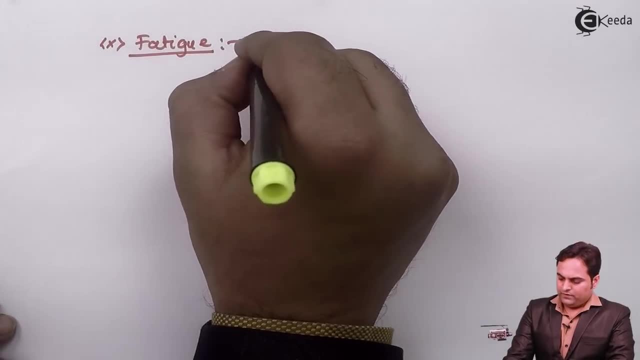 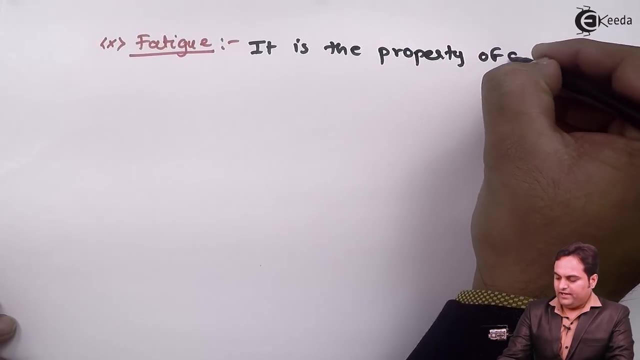 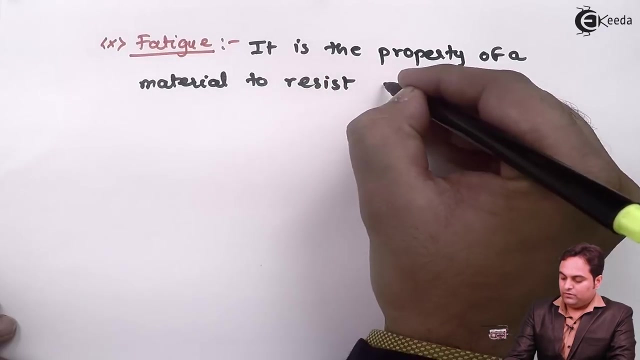 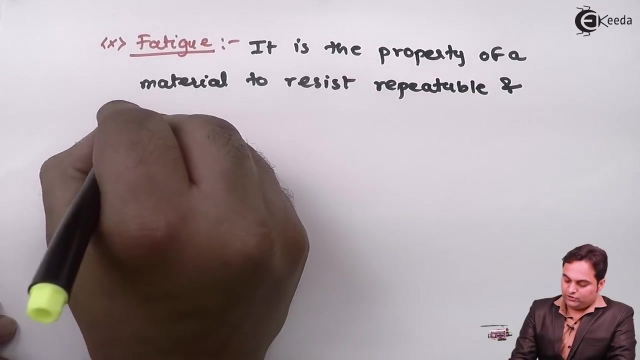 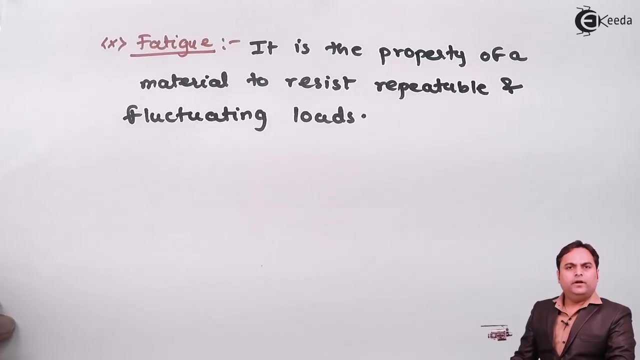 failure. I can say that in case of fatigue, it is the property of a material to resist repeatable and fluctuating loads. it means if we have a machine or an element on which the load is repeatable, that is, it is repeated in a cycle and also it is fluctuating, the load is. 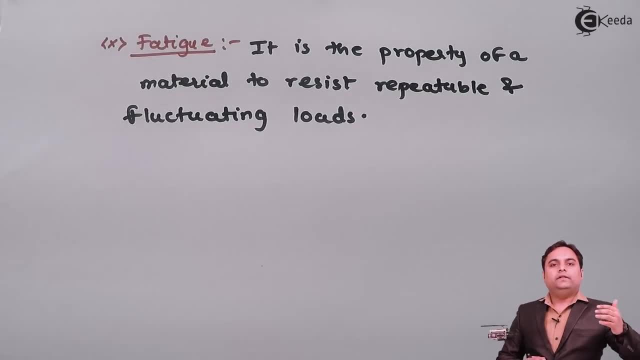 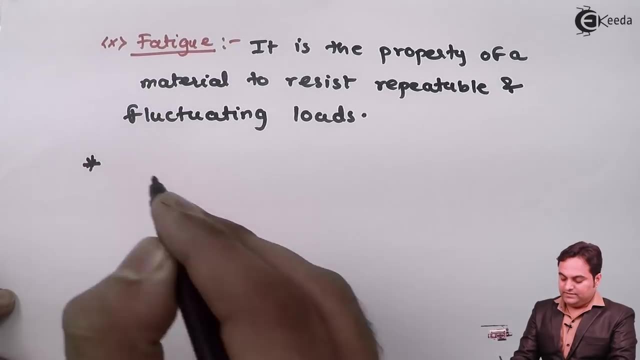 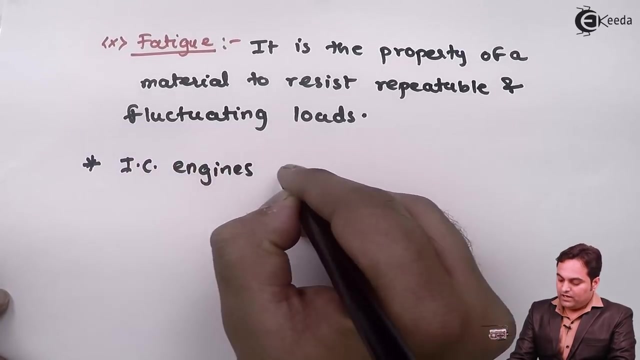 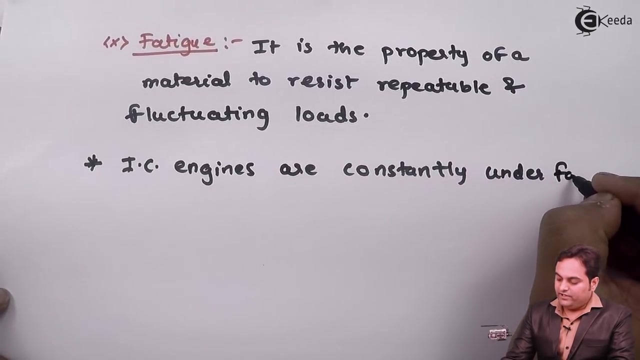 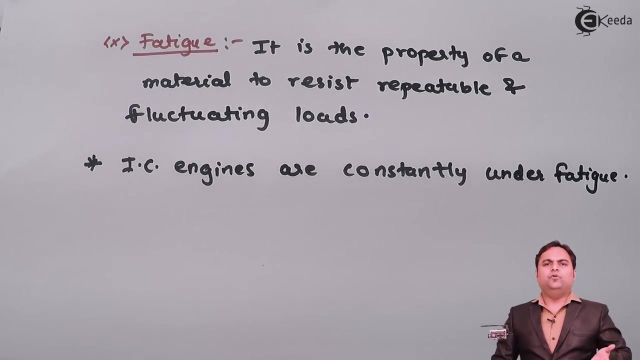 constantly changing from minimum value to maximum value, then what happens? the material would be fatigued and it will break. so here i can say that IC engines, that is internal combustion engines, are constantly under fatigue, because in internal combustion engines the piston is continuously moving temperature, at first during the suction stroke, the temperature is less during compression. 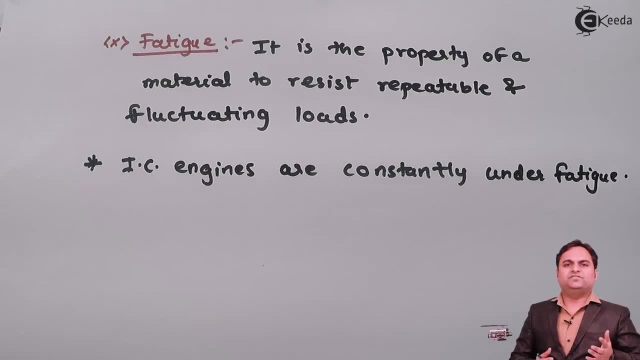 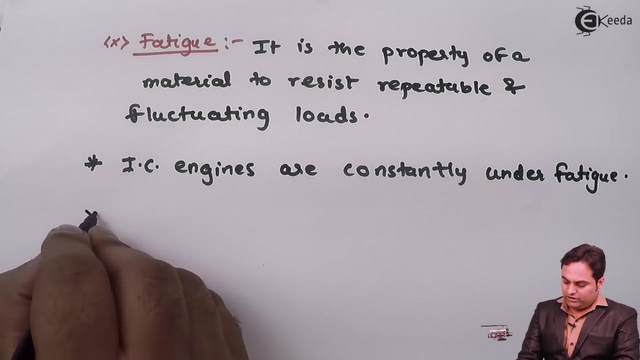 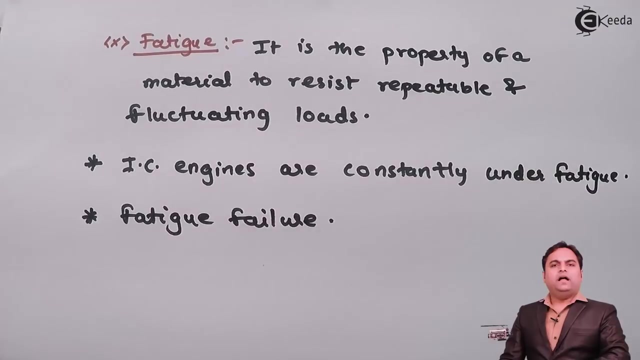 it increases. during the power stroke the temperature is highest and during the exhaust the temperature again decreases. so when it is subjected to continuous variation in load and temperature, that results in fatigue and because of that, the failure which takes place. it is called as fatigue failure and this, the common example which i can give, a fatigue failure is, as i 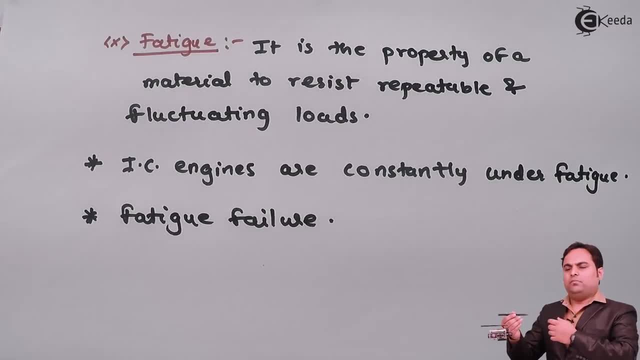 have demonstrated. suppose i have a very thin material or a very thin rod and if i want to break that, then the simplest method is to break it by twisting and untwisting, continuously, applying the load in the opposite direction, and because of that fatigue the material will break. so that is. 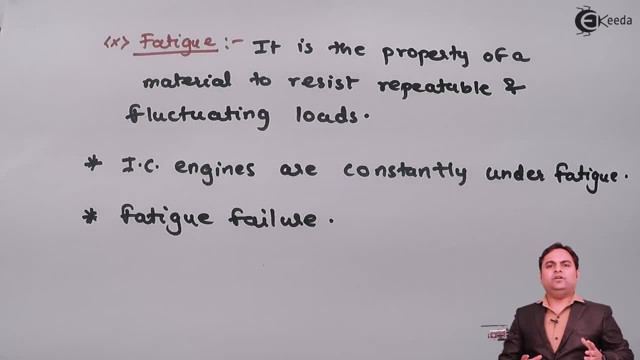 regarding the fatigue failure. so in this video we have seen all mechanical properties in detail.